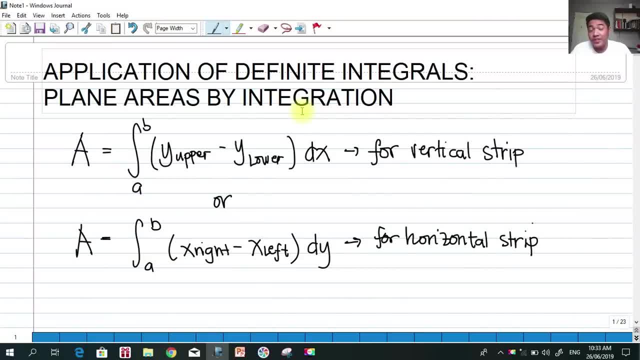 Hi. so for today we're going to talk about the application of definite integrals, more specifically plane areas by integration. So we can use also definite integrals for finding the areas of a plane of a two-curve- okay, in an x-y coordinate. So we have two methods of finding the area of the. 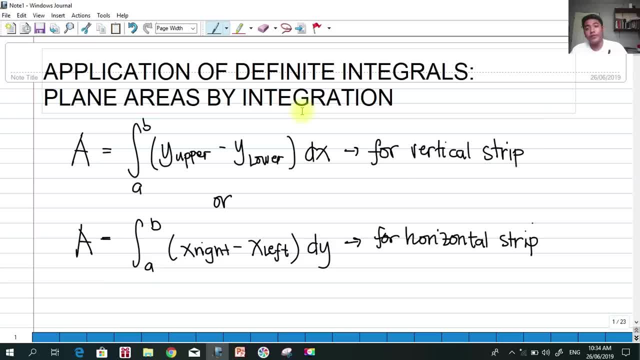 bounded by the two curves, or one curve for the x-axis and one curve for the y-axis, bounded by these two coordinates, or x and y. So for areas we have two formulas. So here we can see that the area is equal to the integral of the so-called y upper minus y lower dx, evaluated from a to b. 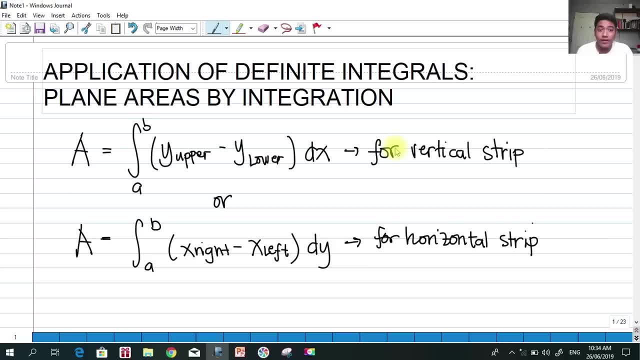 if we're going to use vertical strip for finding the area. Okay, for horizontal strip, we have this following formula: We have this formula. We have a is equals to the integral of x right minus x left, dy evaluated from a to b. So what does this y upper and y lower mean? So we have to express: 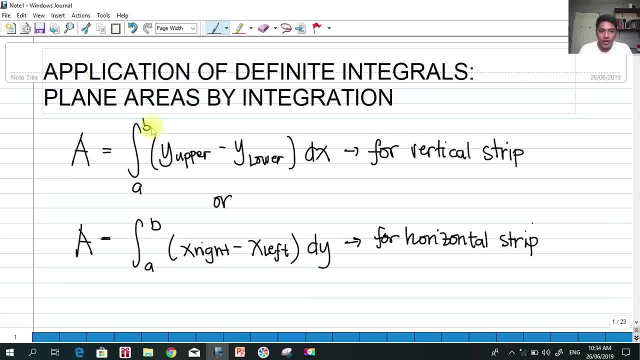 the curve purely in terms of y. So we have to isolate y, okay, in the equation and express it, of course, all in x, so that we can integrate with respect to the x. So what is this? y upper and y lower? Well, actually, that y upper and y lower will depend, okay. 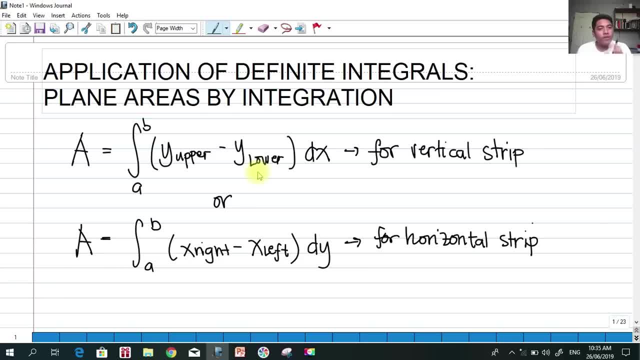 on whether which one of the curve is at the upper side and which one of the curve is on the lower side when we draw a vertical strip. So vertical strip looks like this. So it's actually a very tiny vertical strip, okay. So yeah, And it has a width okay of dx For vertical strip. 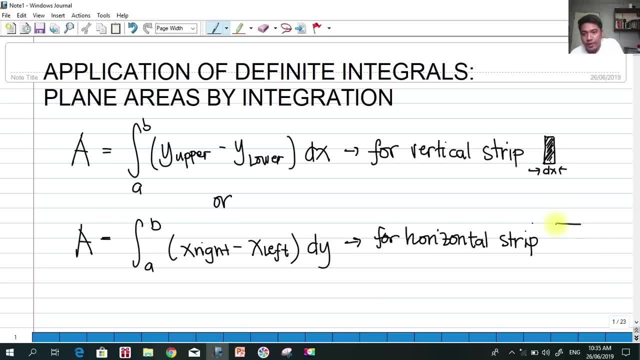 here is what we will use For horizontal strip. I mean Horizontal strip. So this will now be our dy, Okay? So, as you can see, here we have two methods, Sir, what are we going to use? Well, it depends on the curve, okay, and it depends also on the given limits or function. 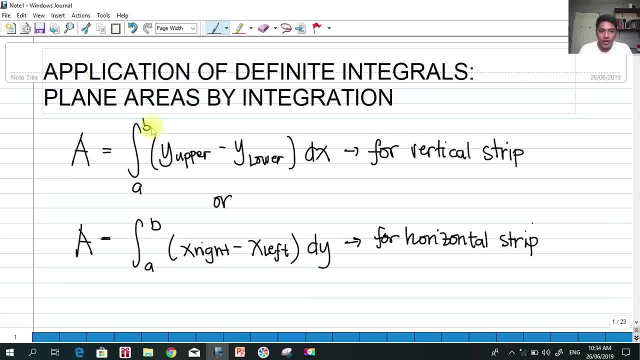 the curve purely in terms of y. So we have to isolate y, okay, in the equation and express it, of course, all in x, so that we can integrate with respect to the x. So what is this? y upper and y lower? Well, actually, that y upper and y lower will depend, okay. 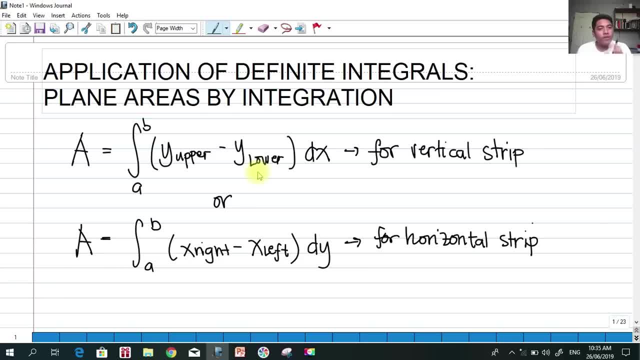 on whether which one of the curve is at the upper side and which one of the curve is on the lower side when we draw a vertical strip. So vertical strip looks like this. So it's actually a very tiny vertical strip, okay. So yeah, And it has a width okay of dx For vertical strip. 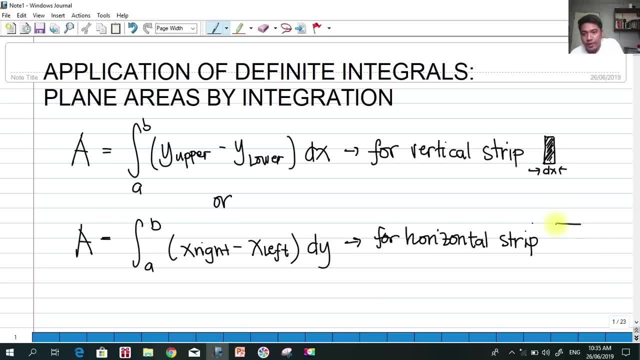 here is what we will use For horizontal strip. I mean Horizontal strip. So this will now be our dy, Okay? So, as you can see, here we have two methods, Sir, what are we going to use? Well, it depends on the curve, okay, and it depends also on the given limits or function. 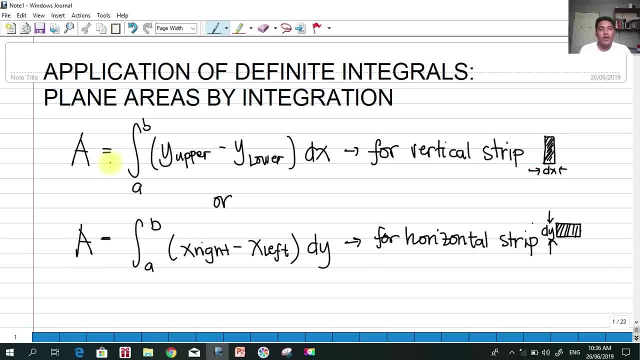 Sometimes the limits are not given from a to b. but if the limits are not given, you have to find the limits. okay, The same as x right and x left. So what are we going to do is to isolate x in the equation and on the other side of the equation, are purely in terms of y, so that we can integrate with. 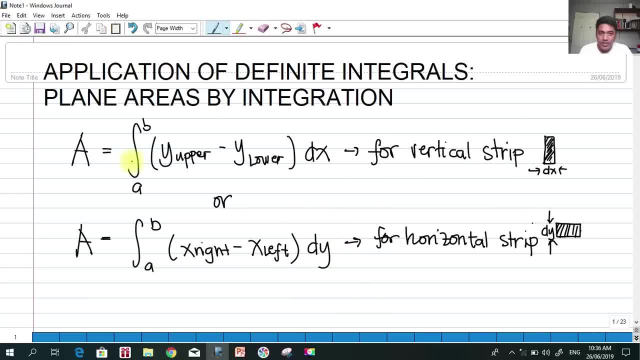 respect to the y. So here are our formulas. Okay, For us to really understand it better, we must try to solve some problems involving this application of definite integral so we can apply these formulas And, again, the rules for finding the areas of the plane along x and y using integrals. 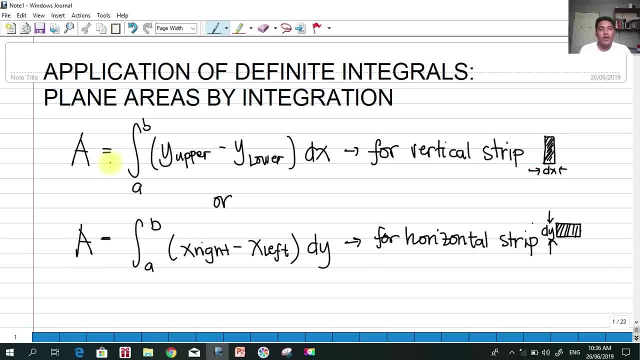 Sometimes the limits are not given from a to b. but if the limits are not given, you have to find the limits. okay, The same as x right and x left. So what are we going to do is to isolate x in the equation and on the other side of the equation, are purely in terms of y, so that we can integrate with. 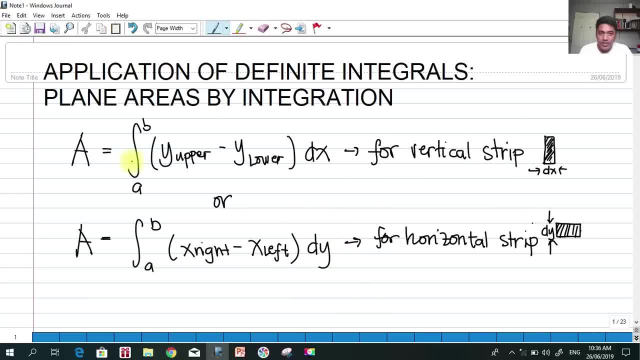 respect to the y. So here are our formulas. Okay, For us to really understand it better, we must try to solve some problems involving this application of definite integral so we can apply these formulas And, again, the rules for finding the areas of the plane along x and y using integrals. 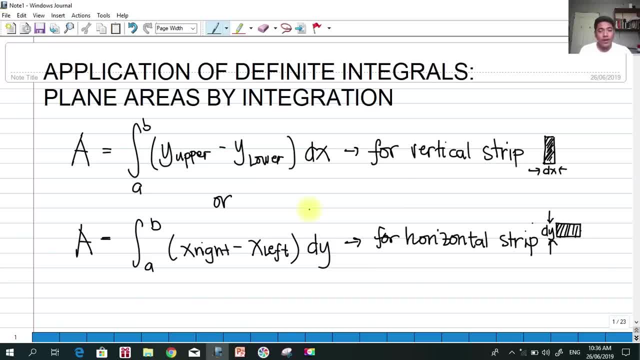 first, you must sketch the given curve, okay, So you must recall the equations of parabola, equations of line whatsoever, given curve, so that we can apply these terms to a particular shelf. So how do you negotiate this? Okay, So, 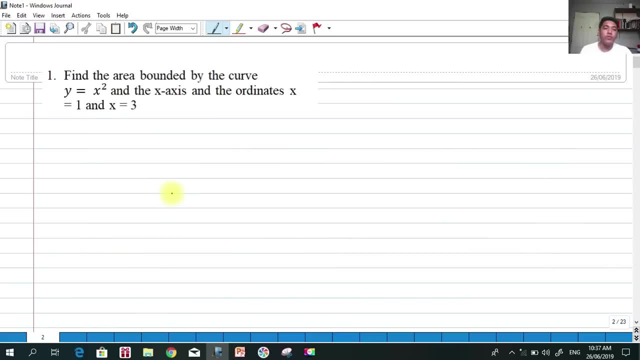 next, we need to separate this part up and count the ensemble force earned form these vectors and the volume of these vectors. Okay, so this is what I'm going to do. Alright, so what I'm actually going to do here is that first I'm going to do the sum of some terms. okay, Let's find now. 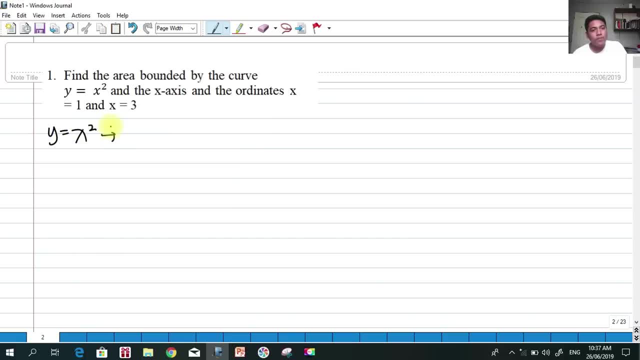 because we're going to do test x now. Okay, and now we're going to find out what the actualρuss is this x slope? Did you know this? Let's find it. Let's find out now, Just find it. sources and the areas by which x is equal to x squared, and the x axis And the coordinates: x is equal to 1 and x is equal to 3.. So first we have to identify this x equal to 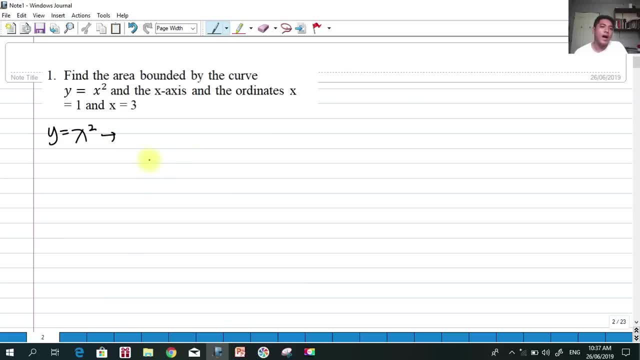 parabola, okay, opening upward, okay. so parabola opening upward, okay, its vertex is at the origin. so what are you going to do? you're going to first make a sketch. okay, make a sketch of that parabola centered at, or vertex at, 0, 0,. so here is our parabola, okay, and 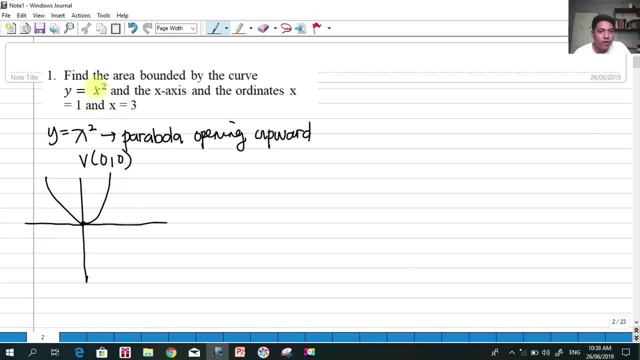 then, okay, it says: find the area bounded by the curve of the parabola and the x-axis. here is the x-axis, okay so, and the coordinates: x is equals to 1, so we have, let's say this: 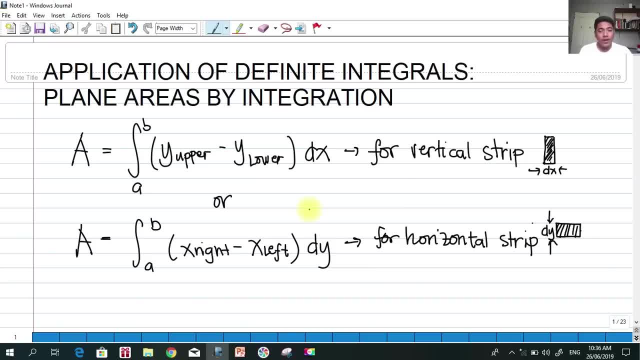 first, you must sketch the given curve. okay, So you must recall the equations of parabola, equations of line whatsoever, given curve, so that we can actually get the area of these curves. Okay So, let's try. So let's try to have 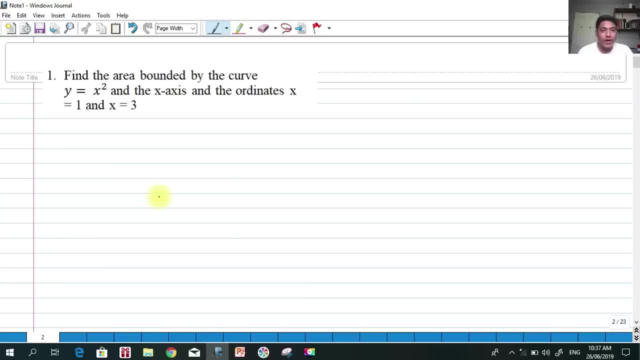 example number one. So find the area bounded by the curve, y is equals to x squared, and the x axis and the ordinate x is equals to 1 and x is equals to 3.. So first we have to identify this: y equals to x squared. 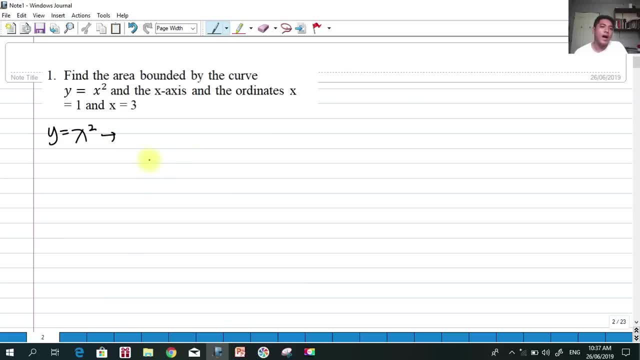 parabola, okay, opening upward, okay. so parabola opening upward, okay, its vertex is at the origin. so what are you going to do? you're going to first make a sketch. okay, make a sketch of that parabola centered at, or vertex at, 0, 0,. so here is our parabola, okay, and 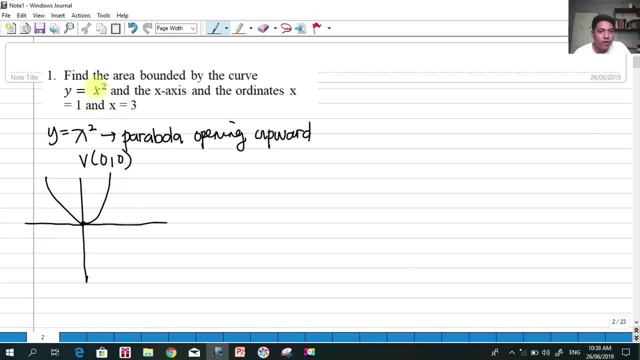 then, okay, it says: find the area bounded by the curve of the parabola and the x-axis. here is the x-axis, okay so, and the coordinates: x is equals to 1, so we have, let's say this: 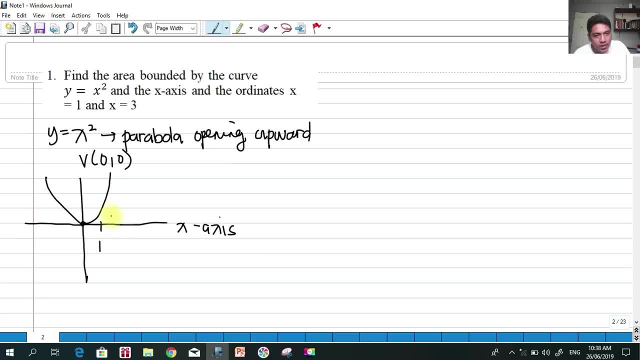 is x is equals to 1, and let's say that this is x is equals to 2.. 3,- okay, my drawing or my label in numbers are not drawn to scale. so it means class. it means that we have to get the area bounded by this parabola, this is our parabola, and 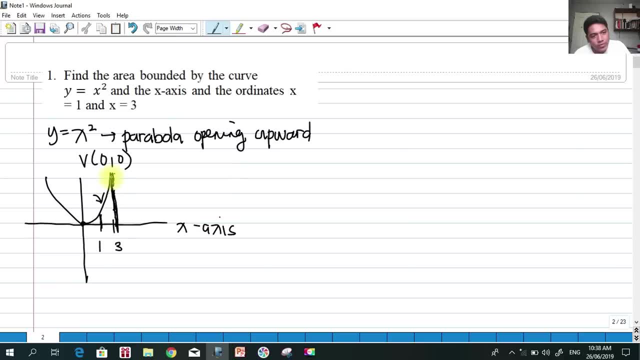 the coordinates x, 1, and 3,. so in this case- oops, in this case- this is the area bounded. okay, Here is the area bounded, so let me just draw it once again. so, for example, this is our. 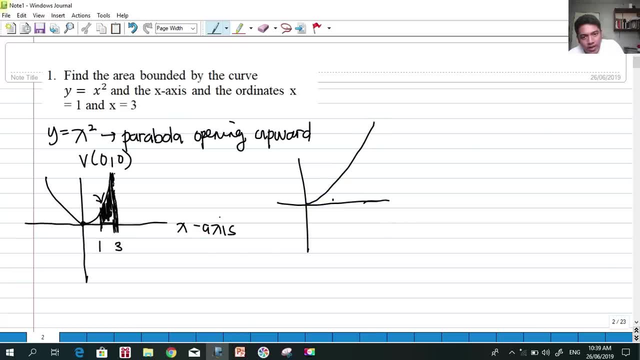 parabola, okay, opening upward. so bounded by x is equals to 1 and x is equals to 3, so, oh, this is our 1 and 3, so what do we do is actually get the area bounded by these? 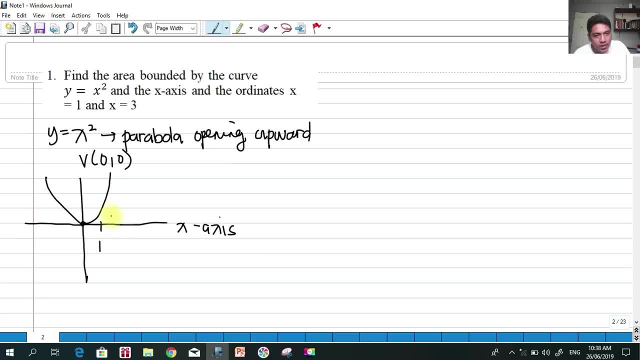 is x is equals to 1, and let's say that this is x is equals to 2.. 3,- okay, my drawing or my label in numbers are not drawn to scale. so it means class. it means that we have to get the area bounded by this parabola, this is our parabola, and 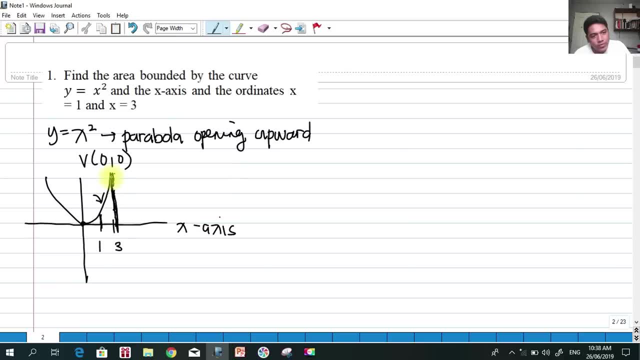 the coordinates x, 1, and 3,. so in this case- oops, in this case- this is the area bounded. okay, Here is the area bounded, so let me just draw it once again. so, for example, this is our. 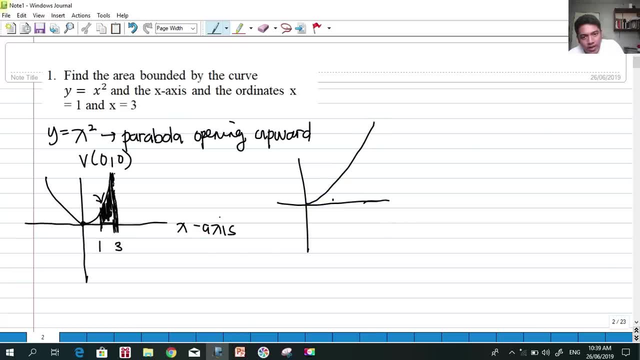 parabola, okay, opening upward. so bounded by x is equals to 1 and x is equals to 3, so, oh, this is our 1 and 3, so what do we do is actually get the area bounded by these? 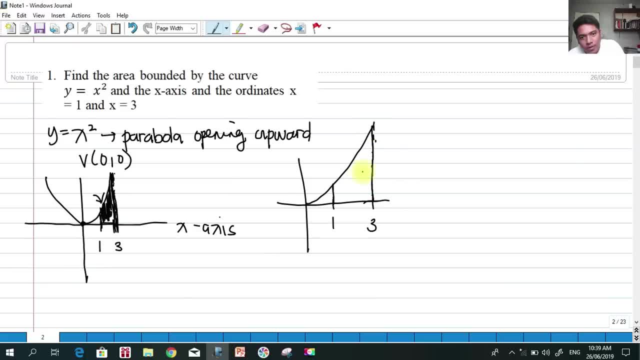 two curves. so this would be our point of of interest. okay, this area, okay. so the question is: what method should we use? Is it a vertical strip or a horizontal strip? So in this problem we can use a. what a vertical strip. so this would now be our vertical. 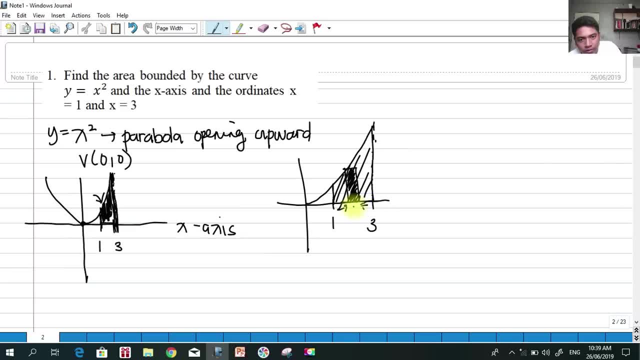 strip. that vertical strip has a length or has a width of dx. so this will now be our: or y is equals to x squared. okay, so the formula again when we use the vertical strip, is: area is equal to the from a to b. so again, what's? what's the formula? 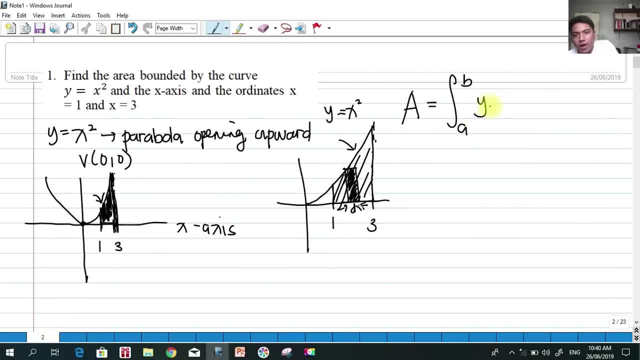 y upper minus y lower, so we have y upper minus y lower dx. okay, Okay, Okay, so we have now this. so, as you can see, if our method is vertical strip, that means dx, so our limits must be on dx. so, as you can see, here the limit to get the 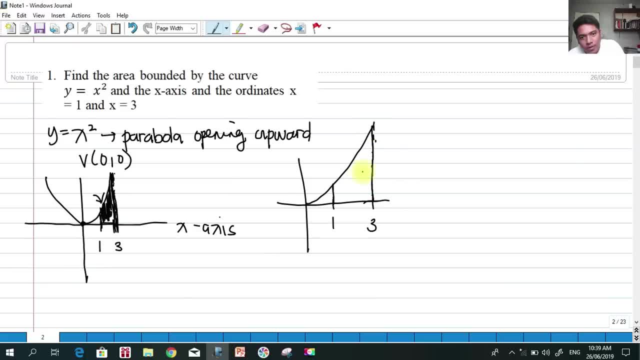 two curves. so this would be our point of of interest. okay, this area, okay. so the question is: what method should we use? Is it a vertical strip or a horizontal strip? So in this problem we can use a. what a vertical strip. so this would now be our vertical. 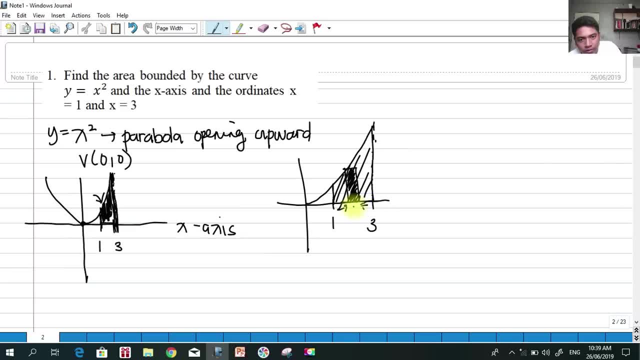 strip. that vertical strip has a length or has a width of dx. so this will now be our: or y is equals to x squared. okay, so the formula again when we use the vertical strip, is: area is equal to the from a to b. so again, what's? what's the formula? 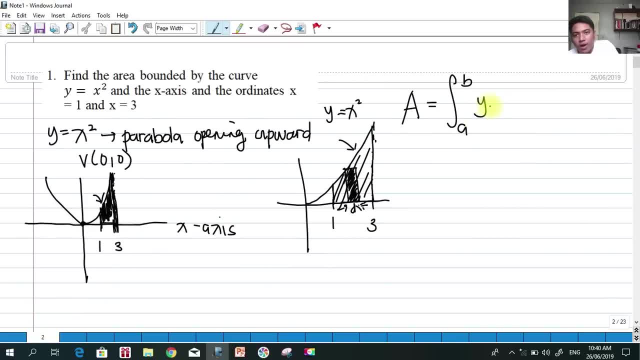 y upper minus y lower, so we have y upper minus y lower dx. okay, okay. So we have now this. so, as you can see, if our method is vertical strip, that means dx. so our limits must be on the x, so, as you can see, here the limit to get the area. 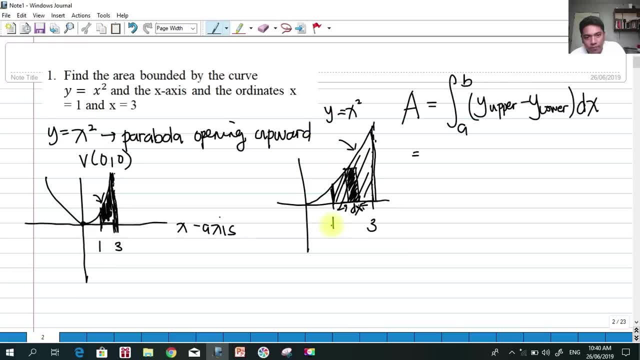 bounded by this okay. parabola and from the coordinates 1 to 3, meaning that should be our limit, from 1 to 3.. Okay, So what is this? y upper and y lower. As you can see here, if you draw this vertical strip, it touches the curve, the parabola. 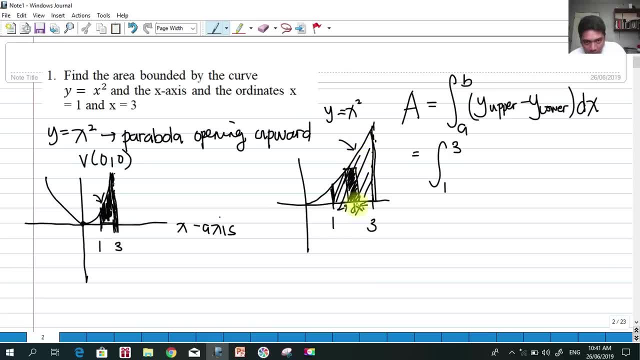 so that should be our y upper, the parabola, and on the lower part of the strip it touches the x-axis. that is not a function, nor that is a curve, so it is simply the axis. so 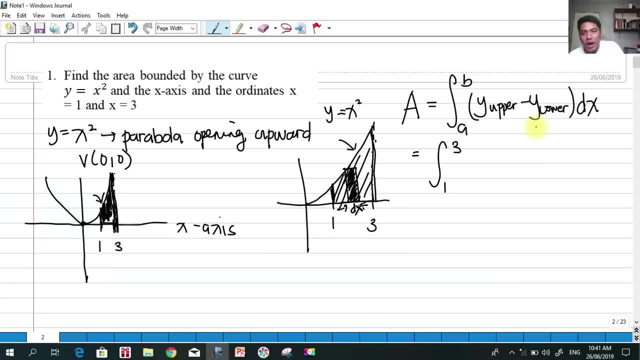 our y lower must be equal to zero. So our y upper. Again, we will express this in terms of isolated y. so we already have this. so y upper will now become x squared. okay, that is our y upper expressed in x. okay, isolated y, that's. 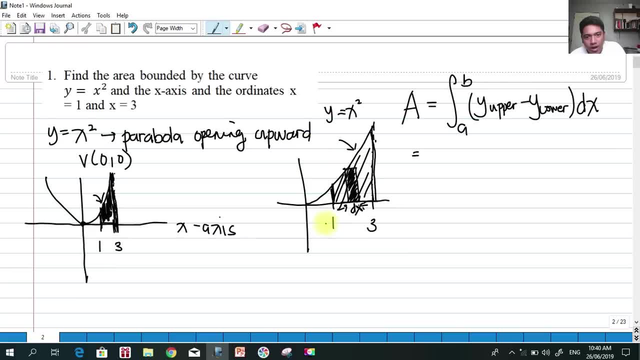 area bounded by this- okay- parabola and from the coordinates 1 to 3, meaning that should be our limit, from 1 to 3.. Okay, What is this? y upper and y lower. As you can see here, if you draw this vertical strip, it touches the curve, the parabola. 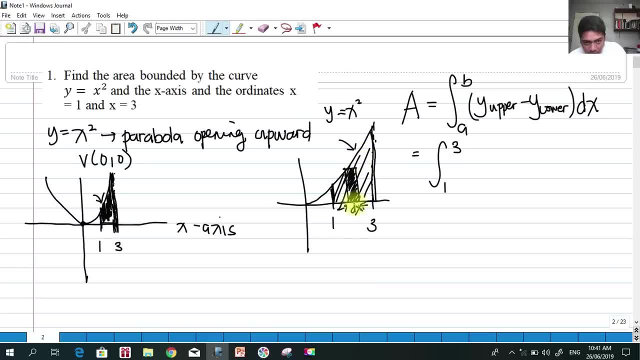 so that should be our y upper, the parabola, and on the lower part of the strip it touches the x-axis. that is not a function, nor that is a curve, so it is simply the axis. so 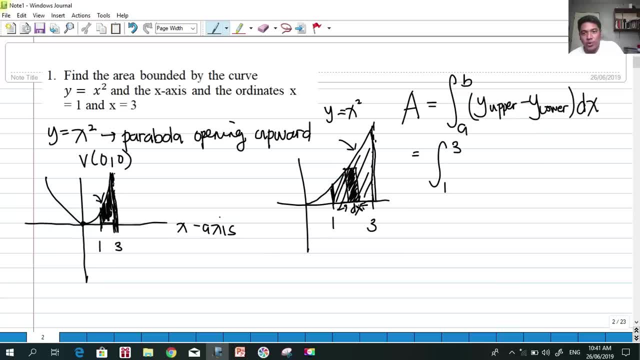 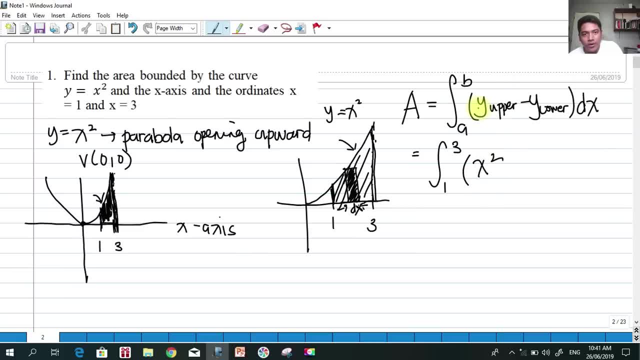 now become x squared. okay, that is our y upper expressed in x. okay, isolated y, that's already isolated, minus the y lower. since it touches the axis x axis, it is zero, so dx. So, simply, we have reduced this formula into x squared, integral of x squared. 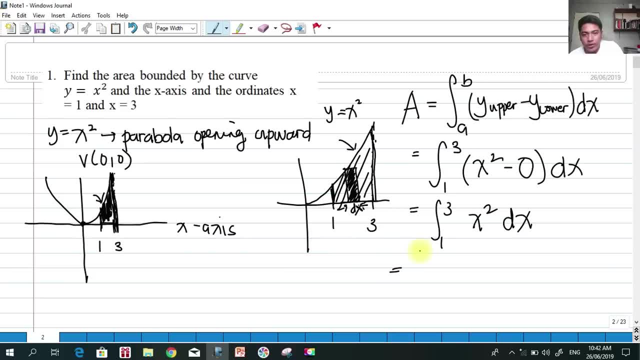 So we know that the integral of this should be x cubed over 3, evaluated from 1 to 3, so that should be 3 cubed over 3, minus, okay, 1. third, so 3 cubed over 3, that is 27 over 3, that 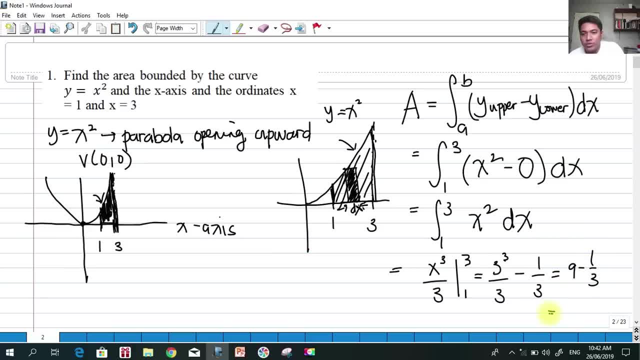 is 9 minus 1 third. okay, this should be 27 minus 1, 26 over 3, that is 9 minus 1 third. so that is 9 over 3 square units. Now, this is the area. okay, this is now the area. our answer for the area. okay. 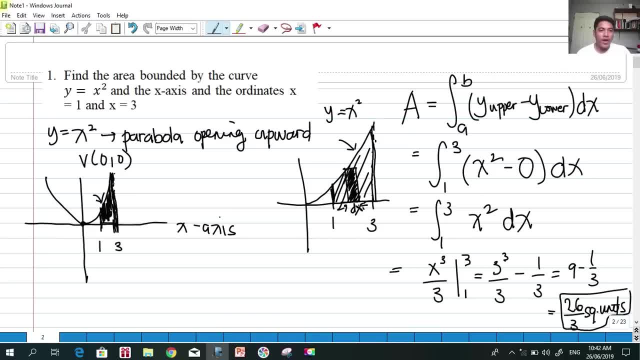 So first we have the graph, the parabola, and then identify the limits. in this case, the limits are given from x1 is equals to x3, and then we use the proper strip for that. in this case, we have used the vertical strip. okay, 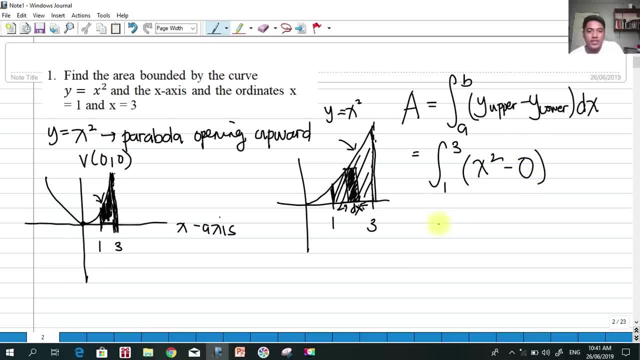 already isolated, minus the y lower. since it touches the axis x-axis, it is zero, so dx. So, simply, we have reduced this formula into x squared, integral of x squared. So we know that the integral of this should be x cubed over 3, evaluated from 1 to 3, so 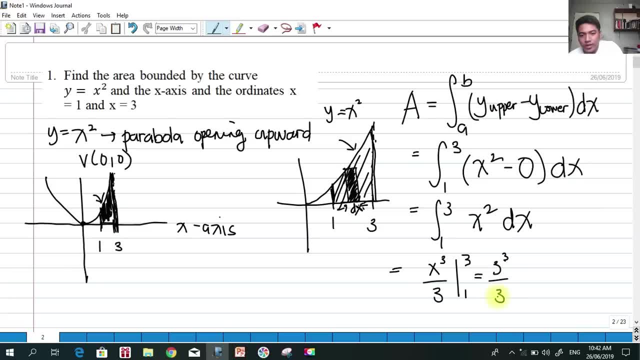 that should be 3 cubed over 3, minus, okay, 1. third. so 3 cubed over 3, that is 27 over 3, that is 9 minus 1. third. okay, this should be 27 minus 1, 26 over 3.. 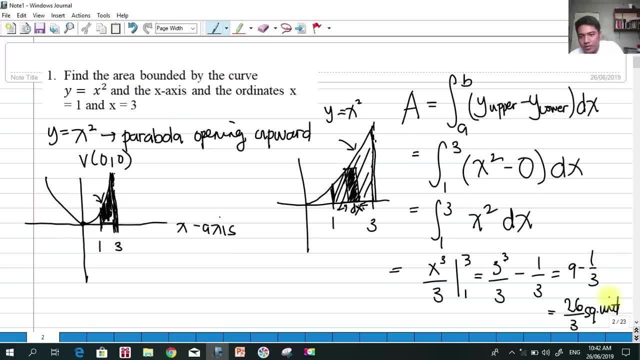 So we have now got the integral of x squared over 3 squared units. This is the area. okay, this is now the area, our answer for the area. okay, So first we have the graph, the parabola, and then identify the limits. 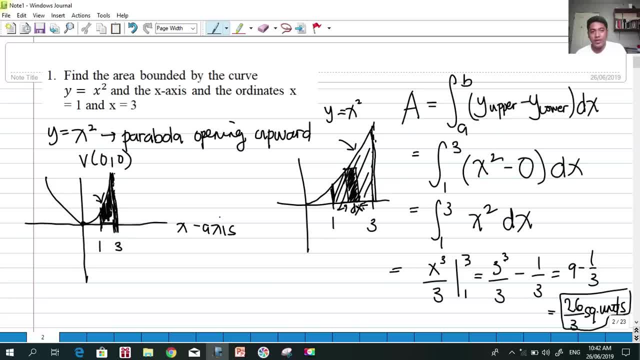 In this case, the limits are given from: x1 is equal to x3, and then we use the proper strip for that. In this case, we have used the vertical strip. okay, Okay, Okay, Okay, Okay, Okay, Okay. 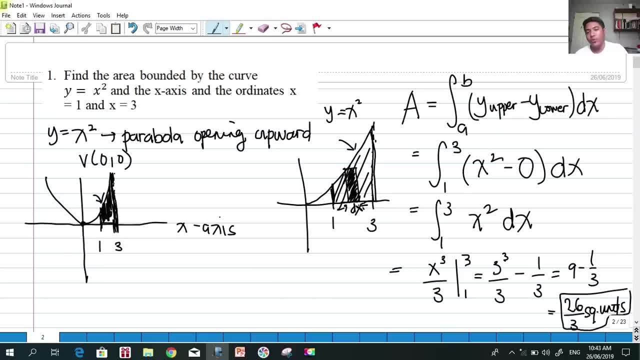 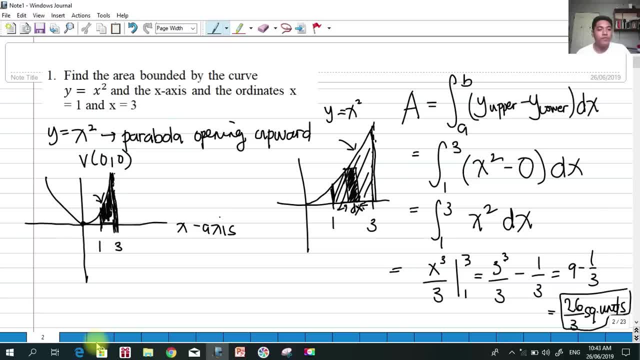 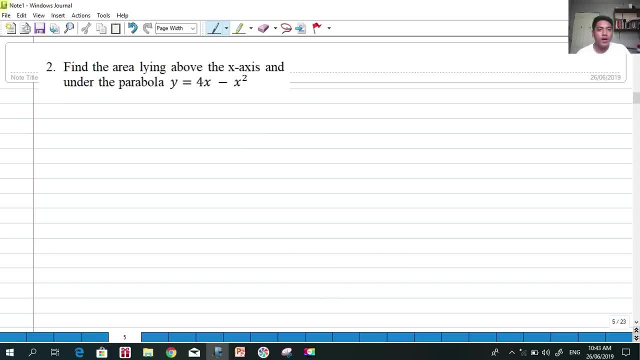 as a negative area. okay, So for number four, number two, find the area lying above the x axis and under the parabola. 4xy equals to 4x minus x squared. Okay, Okay, Okay, first we have to identify what is the opening of this parabola and, at the same time, the vertex of. 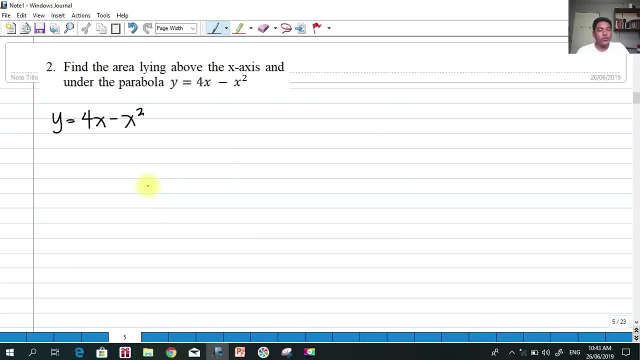 this parabola, okay, so what we're going to do. so first we can rewrite this as negative: x squared plus 4x- okay. we can factor out negative. so x squared minus 4x- okay, and that is equal to y. so y would now be equal to the negative if we perform completing the square here. 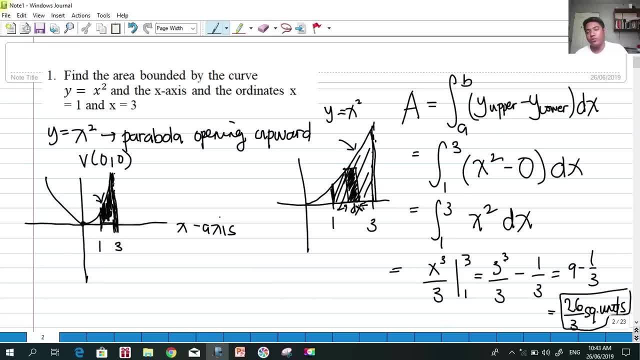 Because we have now the limits: from x is equals to 1 to x is equals to 3.. So we have the answer: 26 over 3 square units. If your answer is actually negative value, that is wrong, Because there is no such thing as a negative area. 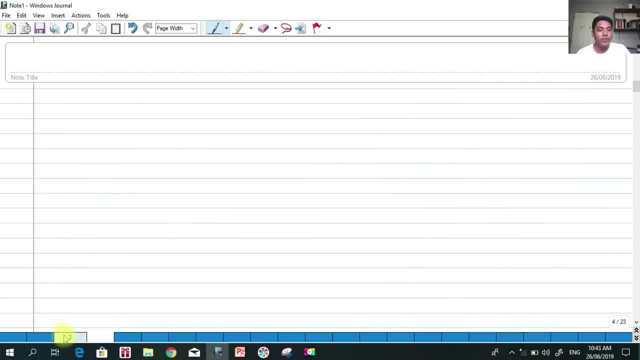 Okay, So for number 2, find the area lying above the x-axis and under the parabola. 4xy is equals to 4x minus x squared. So first we have to identify what is the opening of this parabola and at the same time the vertex of this parabola. 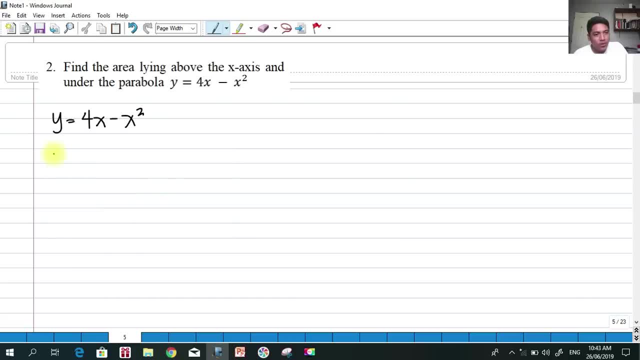 Okay. So what are we going to do? So first, we can rewrite this as negative: x squared plus 4x- Okay. We can factor out negative, So x squared minus 4x- Okay, And that is equal to y. 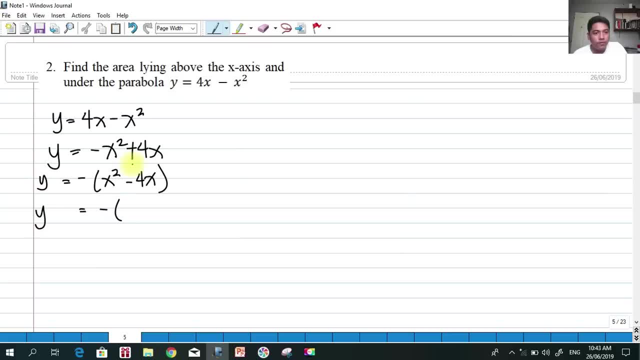 So y would now be equal to the negative. If we perform- If we perform completing the square here, what will happen? So divide this by 2, it would become negative 2.. And then you square the negative 2, that would be plus 4.. 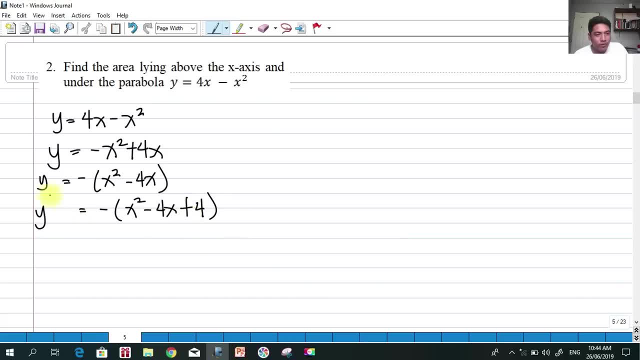 Okay. So, and if we add 4 here, we must also add 4 here on the other side of the equation. But take note, we have a negative here. So technically, when we add 4 here, we are actually subtracting it by minus 4.. 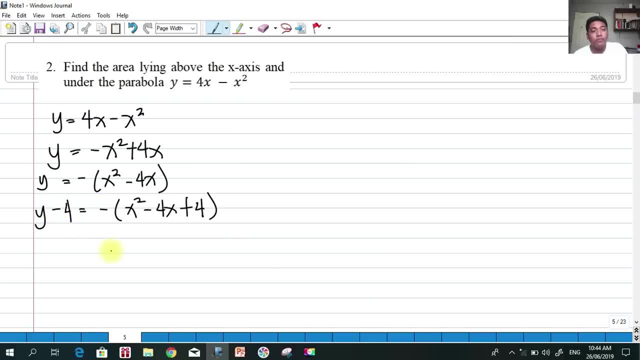 So here we will subtract it. We will subtract it with minus 4, even though we add plus 4 here, because we have a negative here. Okay, And then y minus 4 is equal to the negative. okay, factored form: x minus 2 squared. 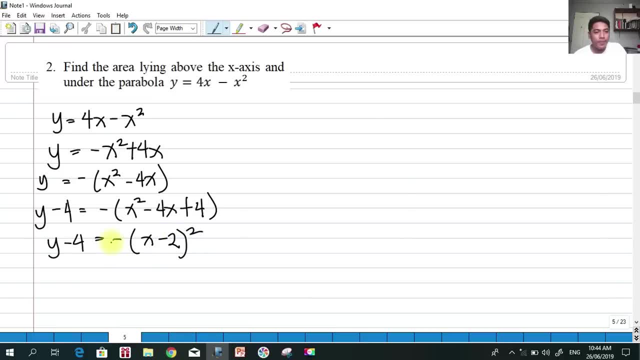 Now, we have now a parabola, okay, opening downward. So we have the vertex of the parabola as 2 and 4.. Okay, This is a parabola opening, So we have the vertex of the parabola opening downward. 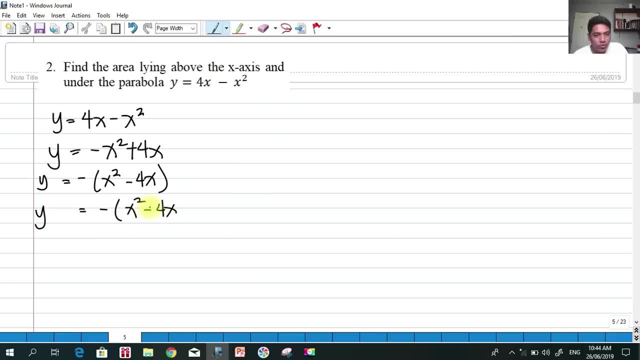 what? what will happen? so divide this by 2. it would become negative 2, and then you're squared: the negative 2, that would be plus 4. okay so, and if we add 4 here, we must also add 4 here, on the other side of the equation. but take note, we have a negative here. so technically, when we add 4 here, 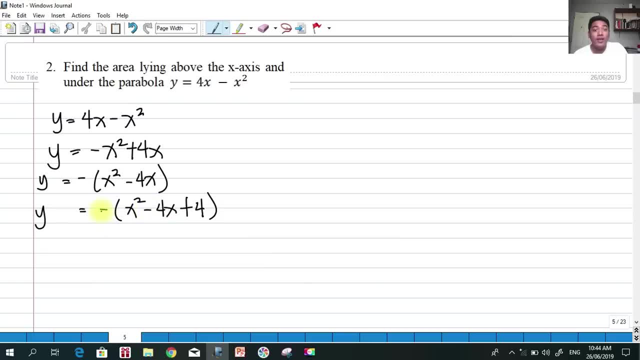 we are actually so subtracting it by minus 4. so here we will subtract it with minus 4, even though we add plus 4 here, because we have a negative here. okay, and then y minus 4 is equal to the negative. okay, factored form: x minus 2 squared now we have now a parabola, okay, opening downward, so we have the vertex of the. 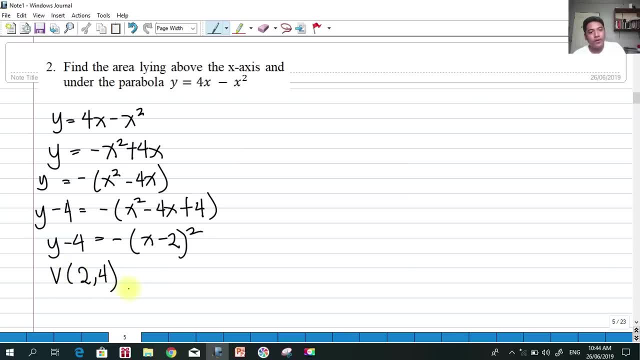 parabola as 2 and 4. okay, this is a parabola opening downward. so the the uh, the shortcut on how are you going to? um? for me, my method to determine uh, what, uh, what is the opening of this parabola is that first take a look at the uh equation. 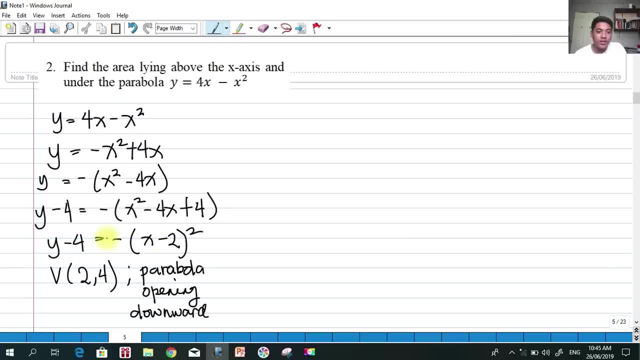 okay, that is a side of the equation that is not squared. in this case that is y minus 4, so y minus 4, y if you, if you see y here. so there is two openings with respect to y: upward and downward. so how will you know if that is downward or upward? you take a look at the sign again of x here, which is a. 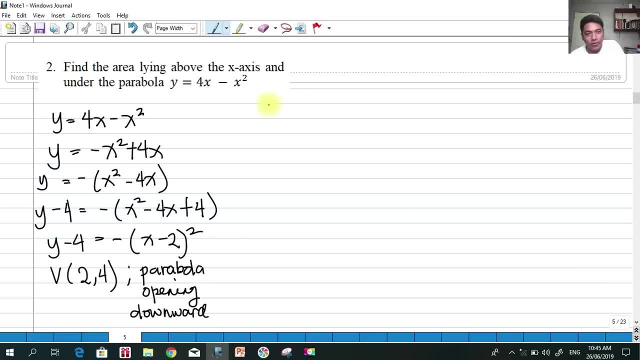 square. so we have a negative here. so it means it's opening downward. so let me just try to draw. i hope i could draw it. so we have the vertex 1, 2, okay, so for y we have, let's say, one, хорошо. 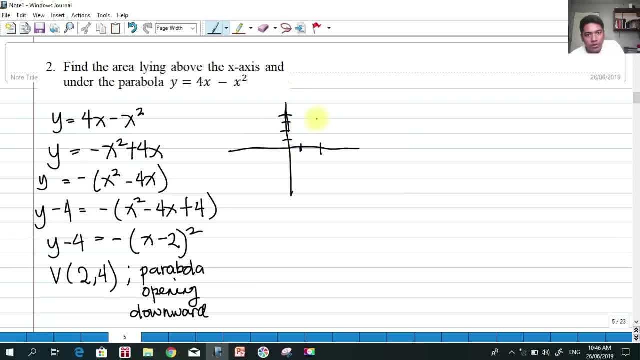 so for y, we have, let's say, one, two, three, four, so that our vertex is here of the parabola and it is actually opening downward. so if i draw a parabola opening downward, it would look like this: okay, this, okay. so this is our x-axis and this is our y is equal to 4x minus x squared. okay, so what? the? 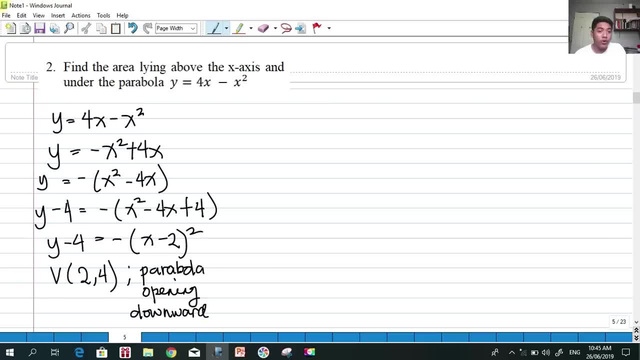 So the shortcut on how are you going to? for me, my method to determine what is the opening of this parabola is that first take a look at the equation. okay, that is side of the equation that is not squared. In this case, that is y minus 4.. 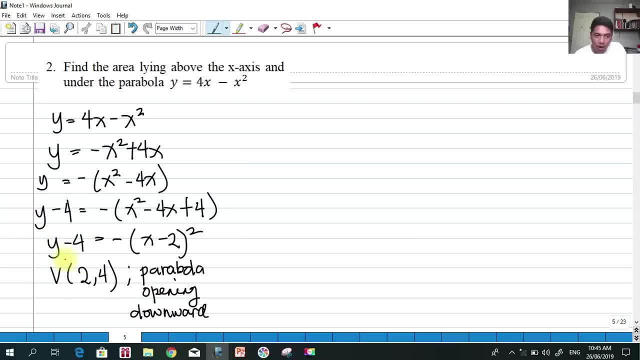 So y minus 4, why, If you see y here? so there is two openings with respect to y, upward and downward. So how will you know if that is downward or upward? You take a look at the sign again of x here, which is a square. 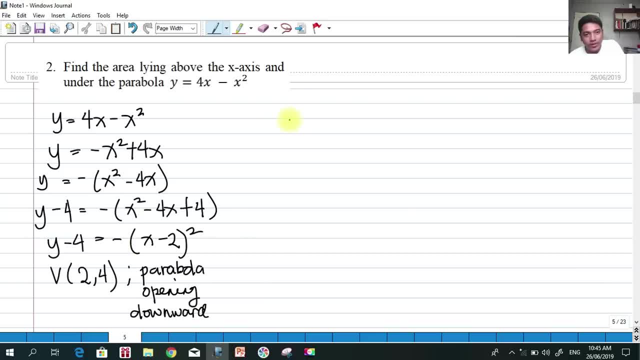 So we have a negative here, so it means it's opening downward. So let me just try to draw. I hope I could draw it. So we have the vertex 1,, 2, okay, So for y we have, let's say, 1,, 2,, 3, 4, so that our vertex is here of the parabola. 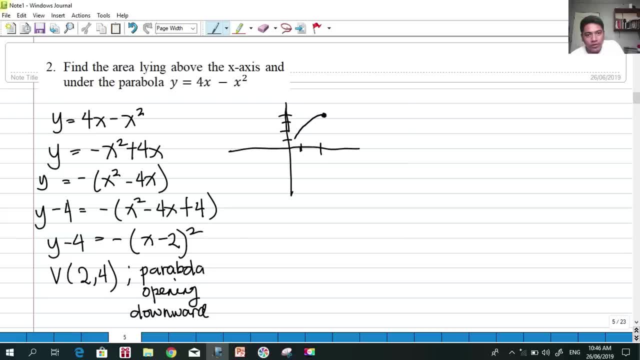 And it is actually opening downward. So if I draw a parabola opening downward, it would look like this: okay, So this is our x-axis And this is our y is equal to 4x minus x squared. Okay, So what the problem is trying to say? find the area lying above the x-axis. 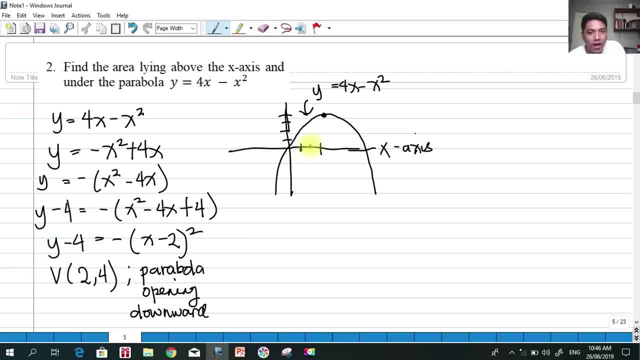 So this is the x-axis, above the x-axis and under the parabola. okay, this So the point of interest. the area we are trying to find is this: bounded by the x-axis, above the x-axis and below the parabola. 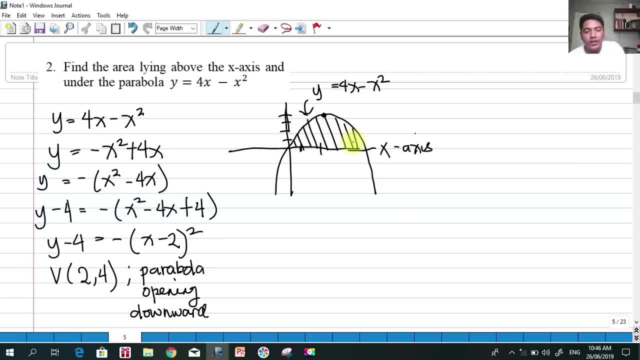 Okay, So we have already drawn, okay, the curve. So what strip are we going to use? Well, of course, Of course, we can use what? still a vertical strip here. okay, We can use still a vertical strip here. 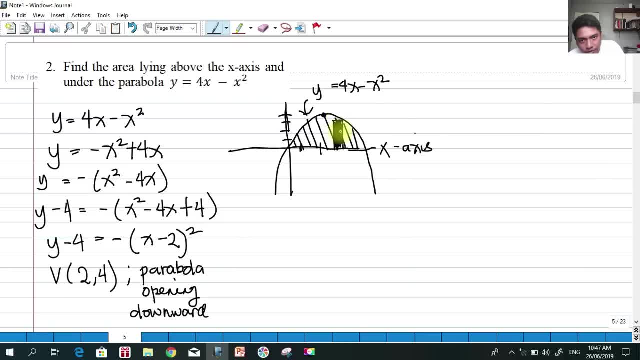 For example, we use a strip here so that this would become our vertical strip And actually its thickness or width is dx. okay, So if we use a vertical strip we have, a is equal to from a to b, y upper minus y lower. 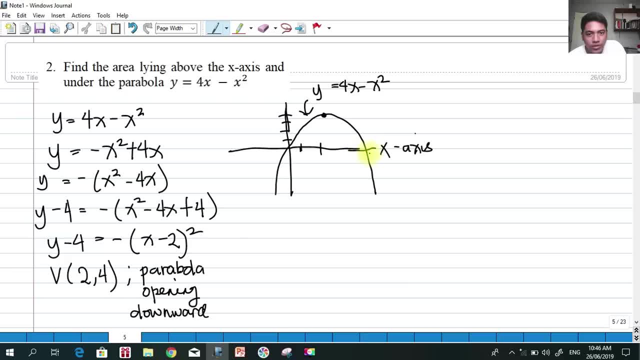 problem is trying to say, find the area lying above the x-axis. so this is the x-axis, above the x-axis and under the parabola. okay, this. so the point of interest. the area we are trying to find is this, bounded by the x-axis, above the x-axis and below the parabola. okay, so we have already drawn. 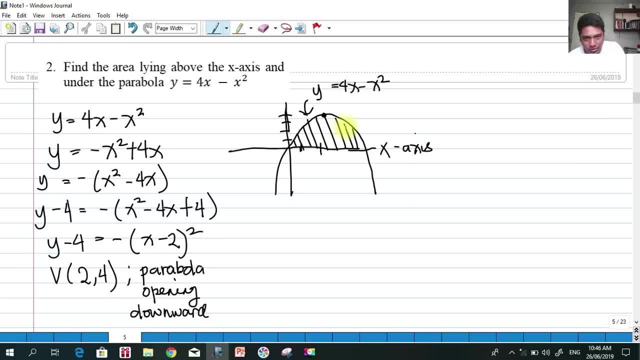 okay, the curve. so what strip are we going to use? well, of course, we can use what- still a vertical strip here. okay, we can use still a vertical strip here. for example, we use a strip here so that this would become our vertical strip and actually its thickness or width is dx. okay, so if you use a vertical strip, we have, a is equals to. 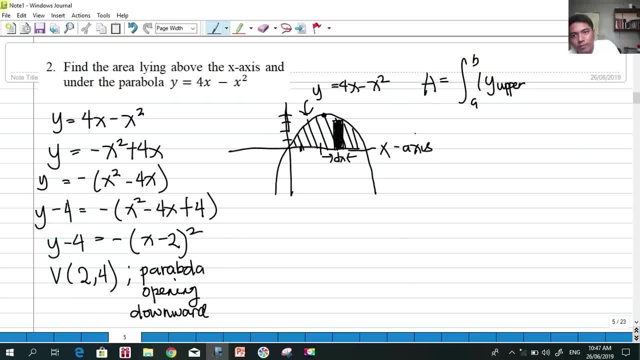 from a to b: y upper minus y lower, uh, dx. okay, that would be our equation, but the problem here is that we don't know the limits a to b. okay, we don't know this. okay, we cannot assume that this is the origin. okay, if we we. 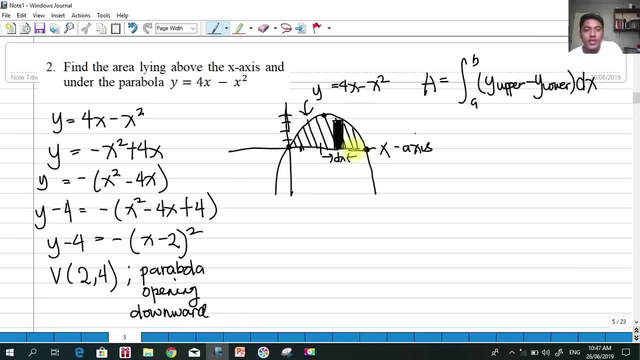 can also have this. so, uh, intersection here. so our limits should be in terms of x, because we have used vertical sleep. so from here to here, that should be our limits, but the problem is that we don't know. so how do we find the limits? simply from the parabola for x minus x squared, oops. 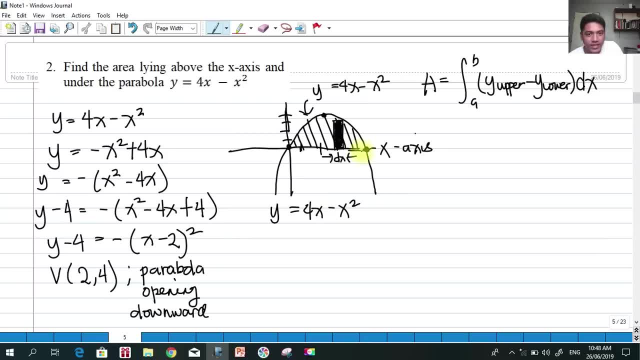 we know that the parabola actually crosses the x-axis, but we don't know exactly what is the point of intersection. so what are we going to do is to equate this y equal to 0 and find the x, so that we can find the limits here to here. so how do we find that? so 0 is equal now to we're. 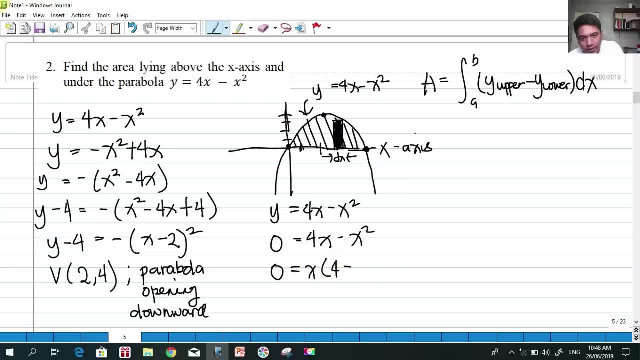 going to factor out x, so we have 4 minus x. so, as you can see here, x is equal to 0, 1x is equal to 0 and 1x is equal to 4.. okay, so the limits, the points of intersection of this parabola with respect to: 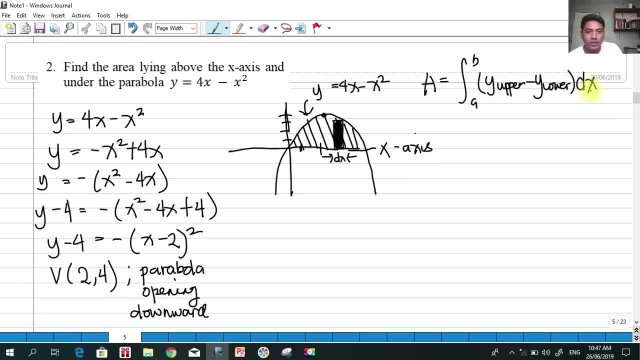 dx. Okay, That would be our equation. But the problem here is that we don't know the limits a to b. okay, We don't know this. okay, We cannot assume that this is the origin. okay, We can also have this. so intersection here. 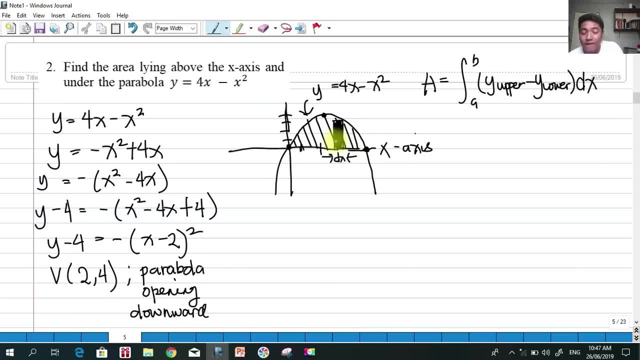 So our limits should be in terms of x, because we have used vertical strip. So from here to here, that should be our limits. But the problem is that we don't know. Okay, So how do we find the limits? Simply from the parabola, for x minus x squared, oops. 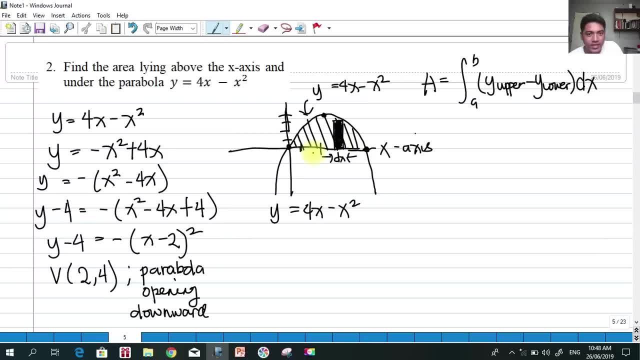 We know that the parabola actually crosses the x-axis, but we don't know exactly what is the point, okay, of intersection. So what are we going to do is to equate this y equal to zero and find the x, so that we 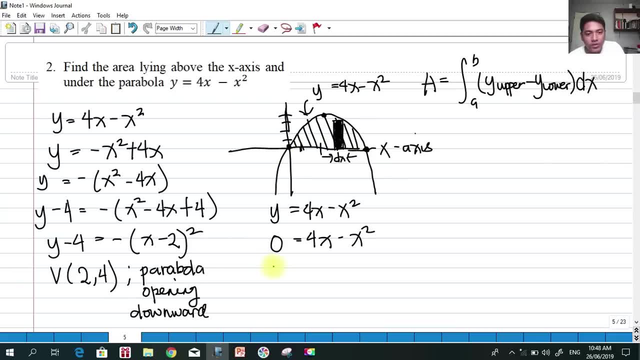 can find the limits here to here. So how do we find that? So zero is equal. now, Okay, We have two, We're going to factor out x, So we have four minus x. So, as you can see, here x is equal to zero, one x is equal to zero and one x is equal. 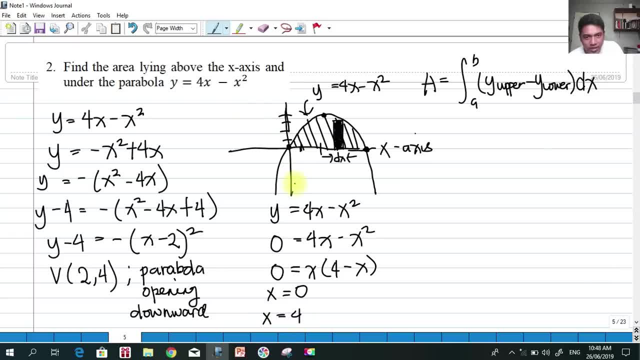 to four. Okay, So the limits, the points of intersection of this parabola with respect to the x-axis should be, according to our drawing, that's correct: zero at the origin and at four. So our limits will now become from zero to four. 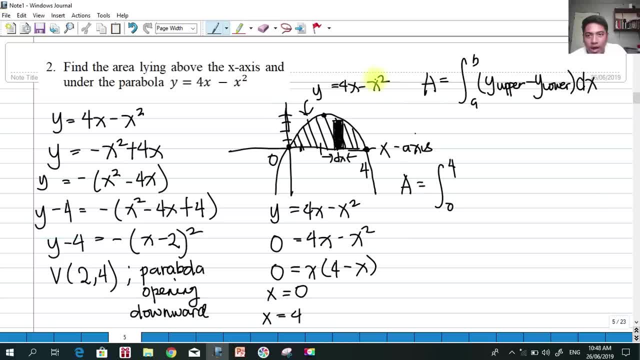 Okay, Again, what is our y-upper? So we have drawn a vertical strip here. It touches the parabola, so that must be our y-upper and it should be expressed in terms of x, because we cannot integrate it if it is expressed in terms of y. 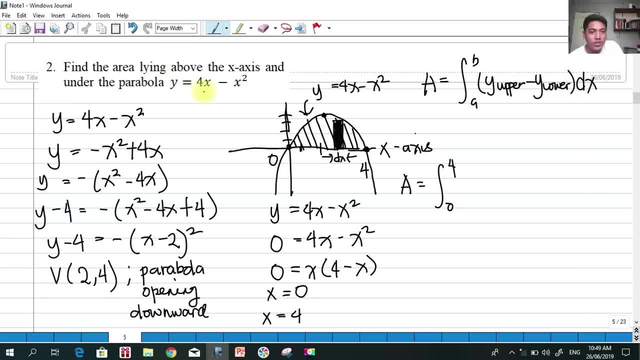 So it's already given. y is already isolated here. so we have four x minus x, squared minus y-lower. The strip touches the x-axis. So that is not equal. Okay, So it means minus zero. So we have a simplification of our formula here. 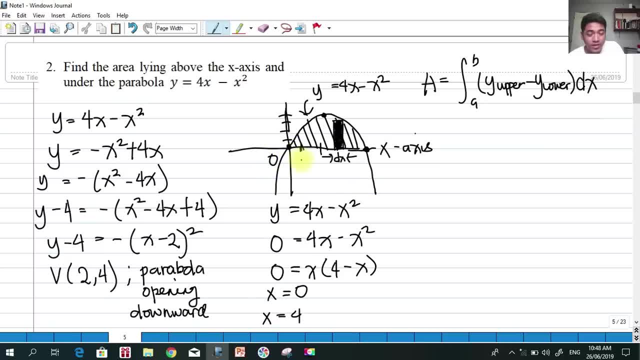 the x-axis should be, according to our drawing, that's correct: zero at the origin and at four. so our limits will now become from zero to four. okay again, what is our y upper? so we have drawn a vertical strip here. it touches the parabola. so that must be our y upper and it should be. 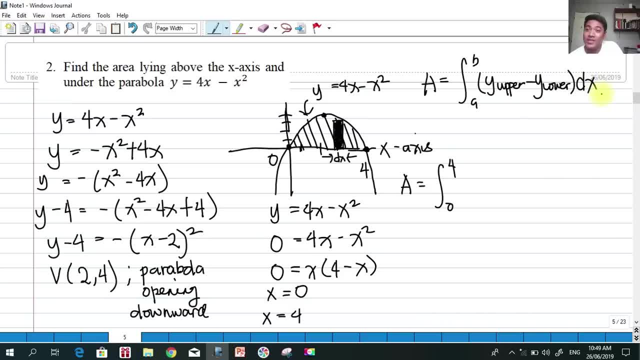 expressed in terms of x, because we cannot integrate it if it is expressed in terms of y, so it's already given, y is also i already isolated here. so we have four x minus x squared, minus y lower, so the strip touches the x-axis. so that is not a curve, so it means minus zero, so we have a. 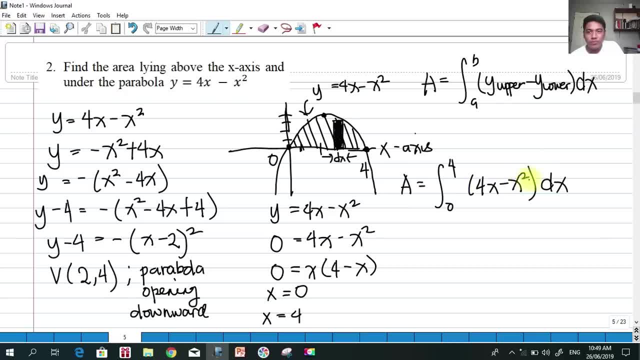 simplification of our formula here. simply, this would be our uh formula. okay, so the area would now be: yeah, okay, if we integrate the x-axis and the y-axis, we have a simplification of our formula. okay, so the area would now be: yeah, okay, if we integrate the x-axis and the y-axis, we have a. 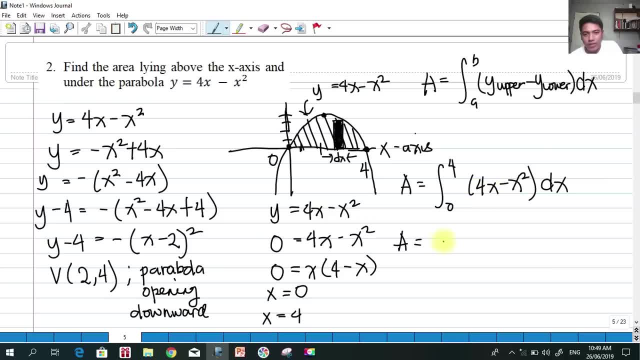 this first: four x squared over two, that should be two x squared, okay, minus one third x cube, with the limits from zero to four. so it turns out that our area would be two times four squared sixteen minus one third four cube, okay. so this should be 32 minus. 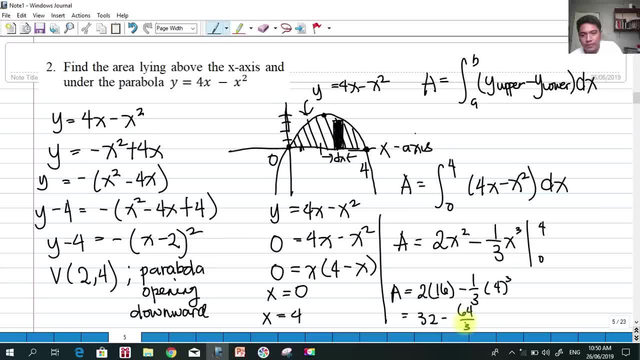 four cube is sixteen. sixty four over three. okay, so if we perform that three times thirty-two, that is, uh, thirty-two times three, six, ninety-six, ninety-six minus sixty-four over three, and ninety-six minus sixty-four is two thirty-two over three square units. so that is the area bounded by. 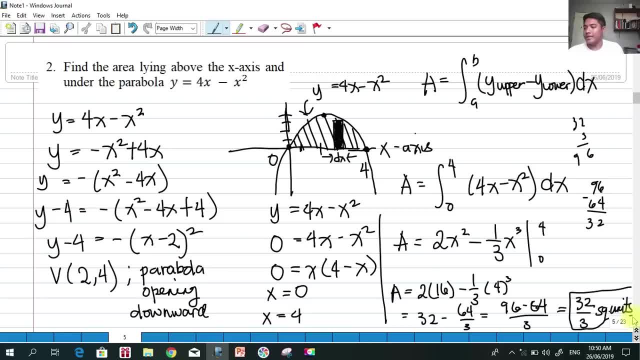 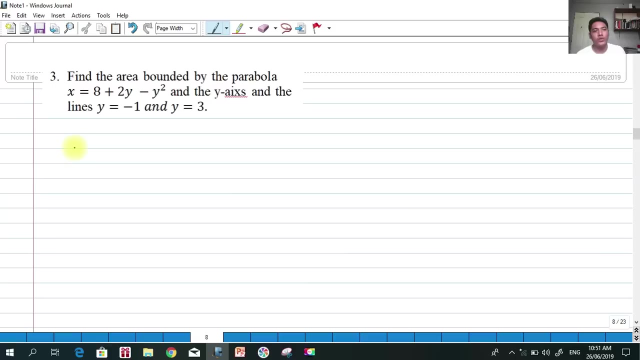 the curve, the parabola and the x-axis. okay, 32 over three square units. okay so, moving on, you can post this video if you uh, actually uh, want to want to review, okay so, but let's try to move on for number three. find the area bounded by the parabola. x is equals to eight plus two, y minus y. 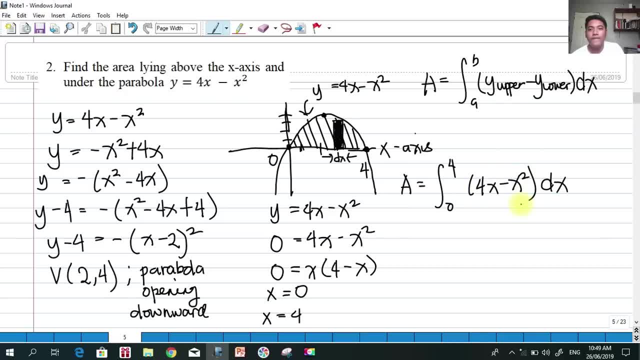 Simply, this would be our formula. Okay, So the area would now be okay if we integrate this first: four x squared over two, that should be two x squared, okay, minus one-third x cubed, with the limits from zero to four. 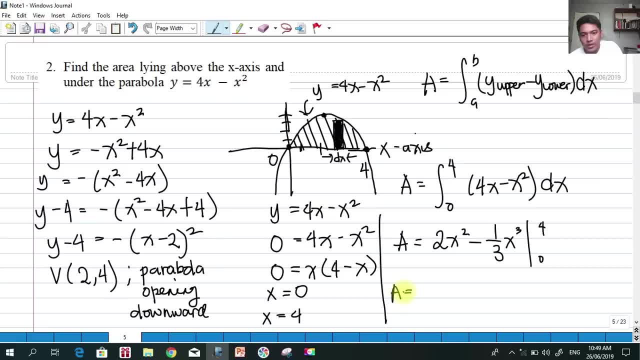 Okay. So it turns out that our area would be two times four squared sixteen minus one-third four cubed. Okay, So this should be thirty-two minus four. cubed is sixteen. sixty-four over three. Okay, So if we perform that three times thirty-two, that is thirty-two times three, six, ninety-six. 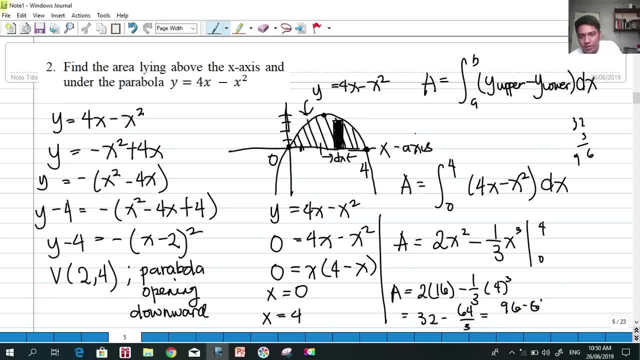 Ninety-six minus sixty-four. Okay, Ninety-six minus sixty-four is two thirty-two over three square units. So that is the area bounded by the curve, the parabola and the x-axis. okay, thirty-two over three square units. 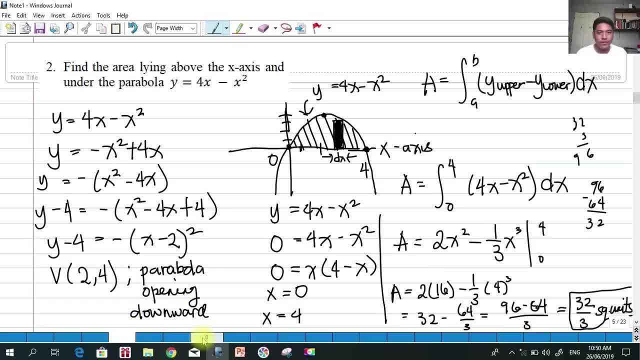 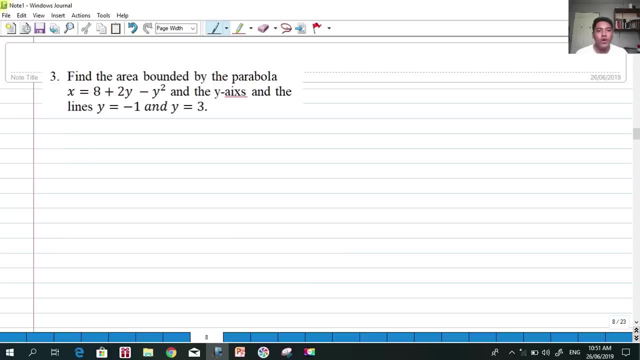 Okay So, moving on, You can post this video if you actually want to review. okay So, but let's try to move on For number three. find the area bounded by the parabola x is equals to eight plus two, y minus y squared, and the y-axis and the lines y is equals to negative one and y is equals. 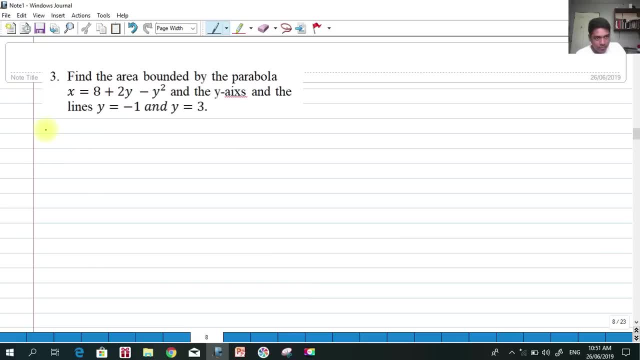 to three. Again, the very first step is we have curves Eight plus two, y minus y squared. This is a parabola. So we can rearrange this equation such that we are going to find the vertex okay and vertex and the opening of this parabola. 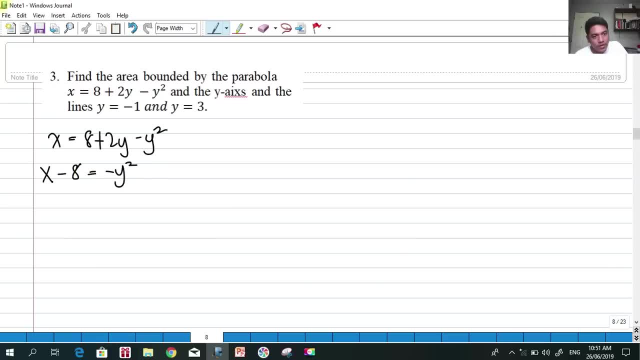 So we have x minus eight minus y squared plus two y. So x minus eight would now be equal to half or half negative y squared. okay, minus two y. Then we're going to perform completing the square here. So y squared minus y squared. 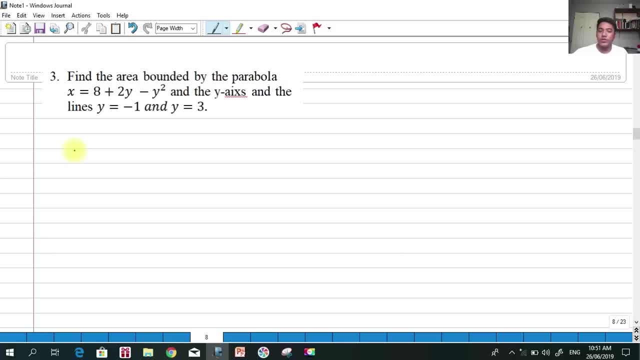 squared, and the y-axis and the lines y is equals to negative one and y is equals to three. again, the very first step is we have verbs eight plus two, y minus y squared. this is a parabola, so we can rearrange this equation such that we are going to find the 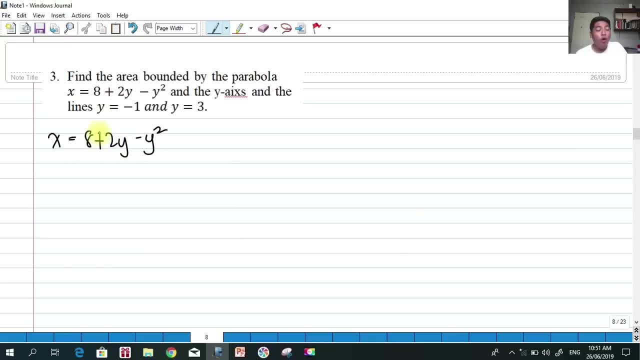 vertex, okay, and vertex and the opening of this parabola. so we have x minus eight minus y squared plus two y. so x minus eight would now be equal to factor out negative. y squared, okay, minus two y. then we're going to perform completing the square here. so y squared minus two, y divided this by two. 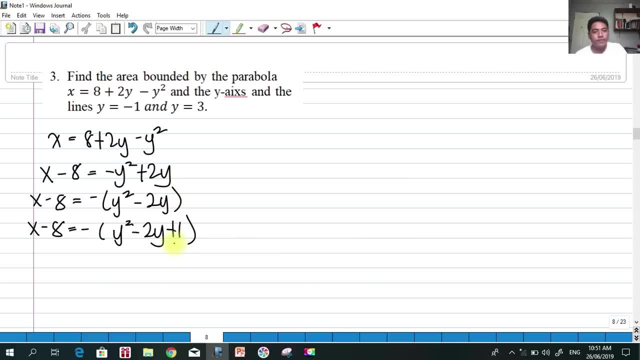 that is negative one. negative one squared would be plus one okay. okay is it. of course, if you added one here, it has a negative sign here. so you must subtract negative one here, such that this would be the left side of our equation. so that should be negative y minus one squared, okay. 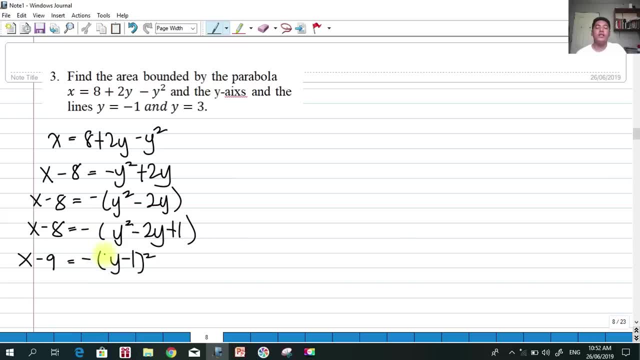 so we have the following: so it is actually a parabola, opening to the left, so opening is left to the left and its vertex is actually on nine and one. okay, nine and one. so if we draw the parabola, we draw the parabola. 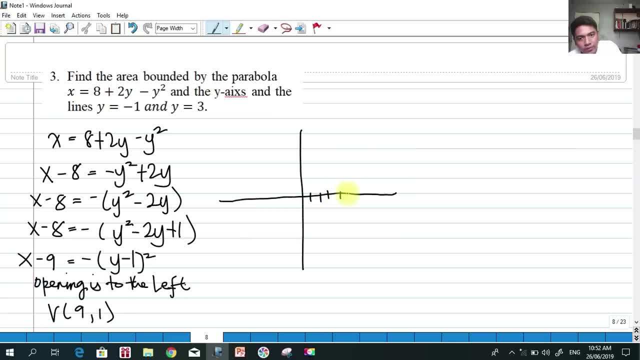 so let's say one, two, three, four, five, six, seven, eight, nine, and this would be the one. okay, so our parabola opens to the left. so this would be the our parabola. okay, forgive me for my drawing. okay, it's not really good, but i'll try my best again. 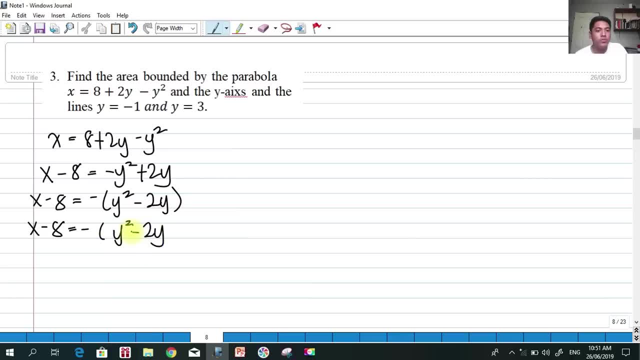 Okay. So y squared minus two. y divided this by two, that is negative one. negative one squared would be plus one. Okay. Okay, Of course, if you added one here, it has a negative sign here. So you must subtract negative one here, such that this would be the left side of our equation. 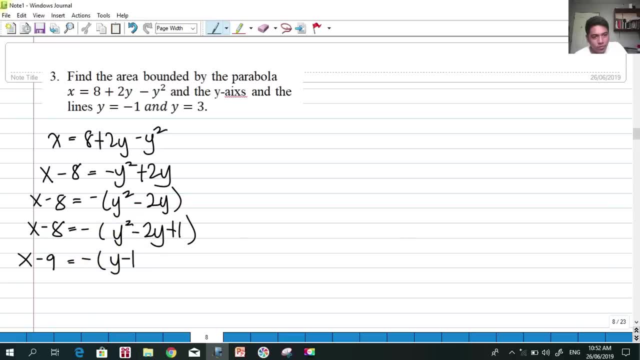 So that should be negative y minus one squared. okay. So we have the following: So So it is actually a parabola, opening to the left. So opening is left to the left And its vertex is actually on nine and one. okay, nine and one. 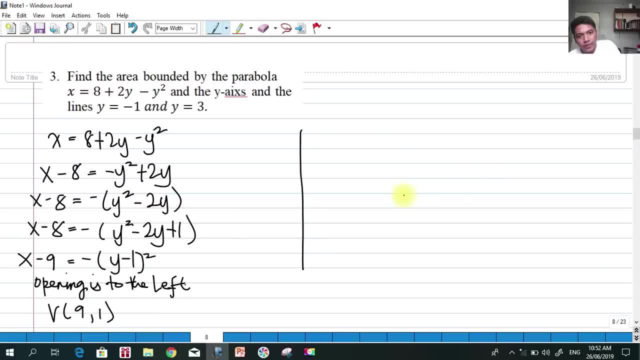 So, if you draw the parabola, if you draw the parabola, Okay, Okay, Okay, Okay. So let's say one, two, three, four, five, six, seven, eight, nine, and this would be. 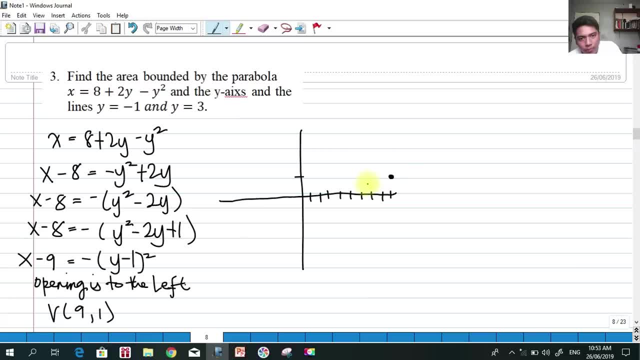 the one. Okay, So our parabola opens to the left. So this would be the our parabola. Okay, Forgive me for my drawing. Okay, It's not really good, but I'll try my best again. 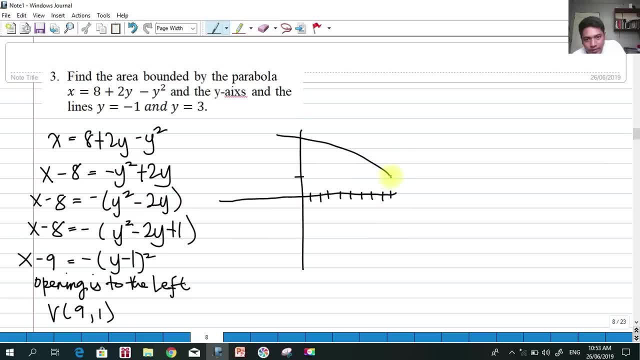 Okay, So let's try to draw. Okay, This should be the parabola. Okay, So that must be our parabola. This is our. y is equals to- or my mistake, that is x equals to eight plus two y minus. 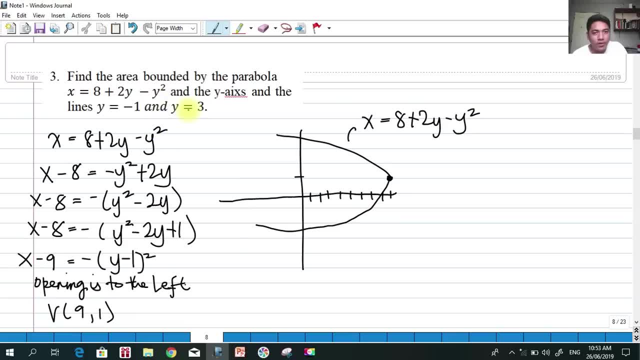 y squared And of course, we have the other given and the y-axis. So find the area bounded by this parabola and the y-axis. This is our y-axis And the lines Y is equals to negative y, Y is equals to negative one. 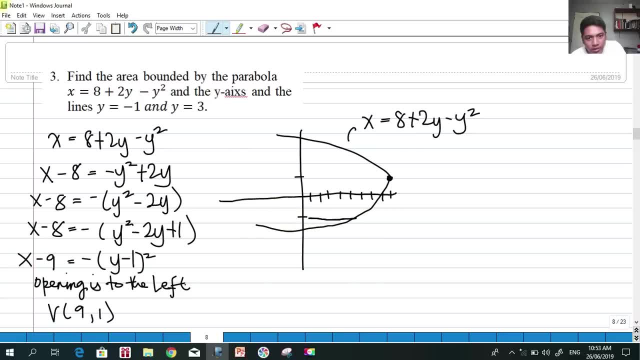 So let's say this is the line that is equal to negative one. Okay, So this is the line. Let's say line y is equals to negative one and the line y is equals to three. Let's say: this is the line that is equal to three. 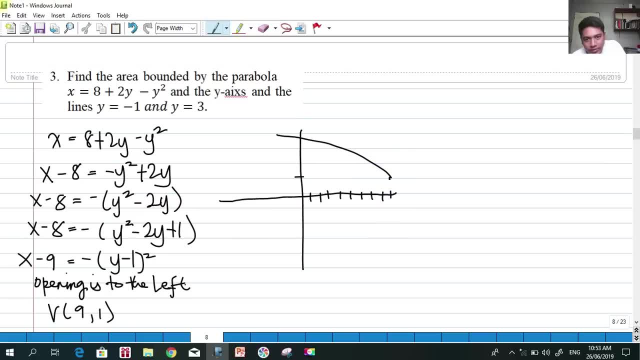 okay, so let's try to draw. this should be the parabola. okay, so that must be our parabola. this is our: y is equals to, or my mistake, that is x equals to eight plus two, y minus y squared. and of course we have the other given and the y-axis. so find the area bounded by. 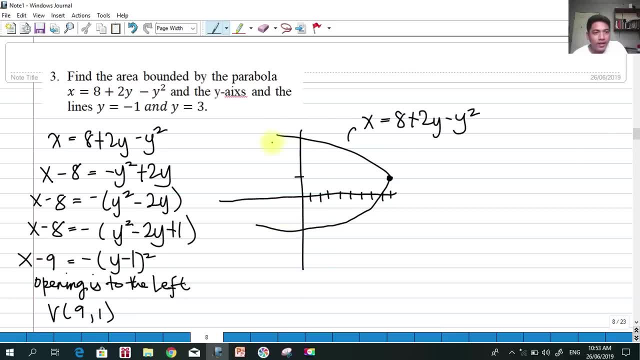 this parabola and the y-axis, this is our y-axis, and the lines y is equals to negative one. so let's say: this is the, the line that is equal to negative one. okay, so this is the line. let's say line y is equals to negative one and the line y is equals to three. let's say: this is the line that. 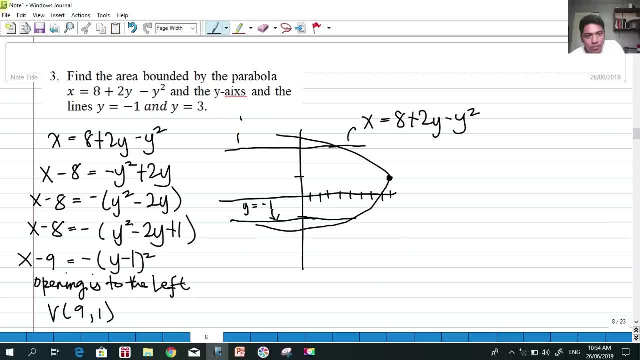 is equal to three. so this is the y is equals to three. so we have two lines here. so the problem is asking: find the area bounded by this parabola, y-axis and the lines. y, c equals to three and y negative one. so our point of interest, the area, is: 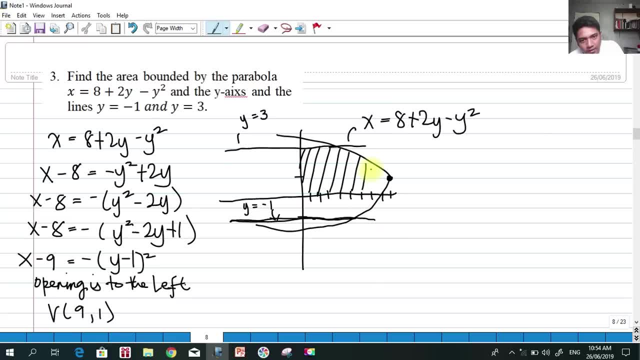 actually what this, this area? well, including the y is equals to negative one. so that much not clear. just saying inlıotto and the y-axis and located by y-axis, so less is equal to three and y-1 theikutive as well. i will do my test. i will do my test. if you don't work, less你. 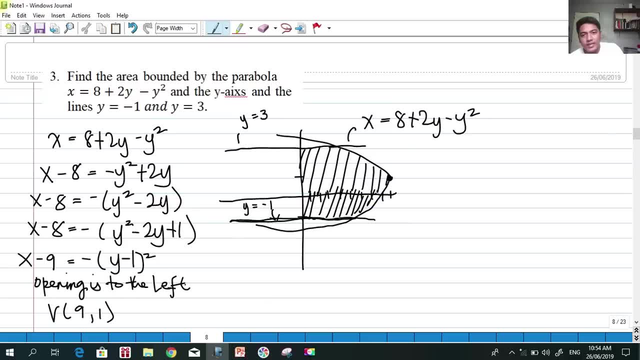 approach by find the area boundary, by, So that must be the area. Okay. So the next step is: what method are we going to use? Okay, What method are we going to use? What strip, So, as you can see here, we can use, since we have the limits from negative 1 to 3,. 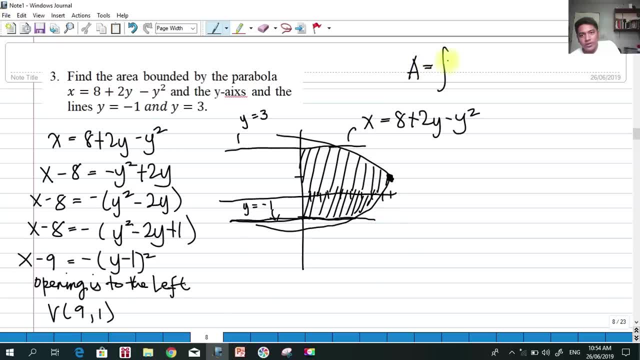 so we can use the what Horizontal strip that is x right minus x left. Okay, dy, from a to b. In this case we will be needing a limit that is in terms of y, that is given from negative 1 to 3.. 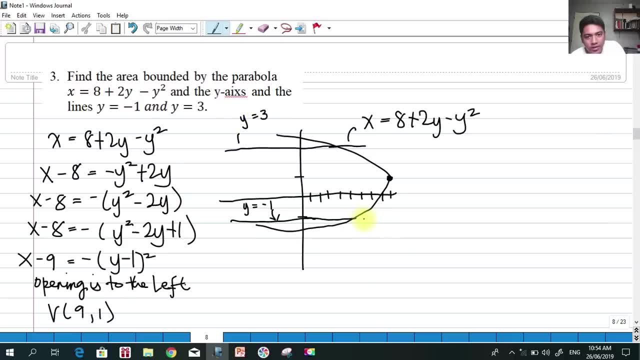 So this is the y is equals to three, So we have two lines here. So the problem is asking: find the area bounded by this parabola. Okay, This parabola, y-axis and the lines y is equals to three and y, negative one. 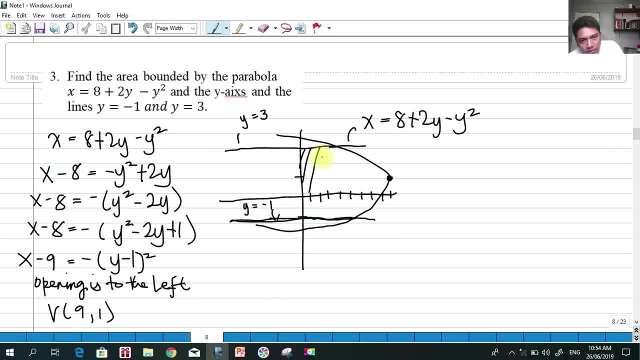 So our point of interest, the area, is actually what? This, This area, Well, including the y, is equals to negative one, So that must be the area, Okay. So the next step is: what, what? okay, what method are we going to use? 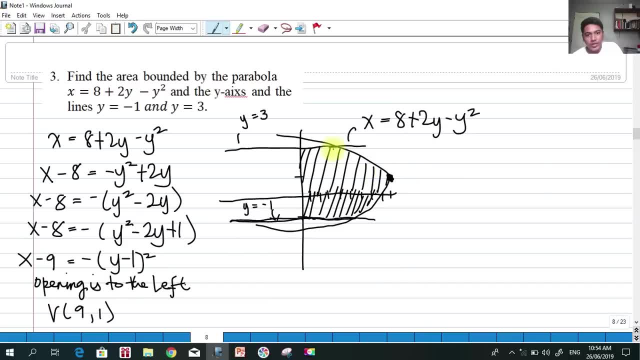 Okay, What method are we going to use? What strip? So, as you can see here, we can use, since we have the limits from negative one to three. so we can use the what Horizontal strip, That is, x right minus minus x left right, dy, from a to b. 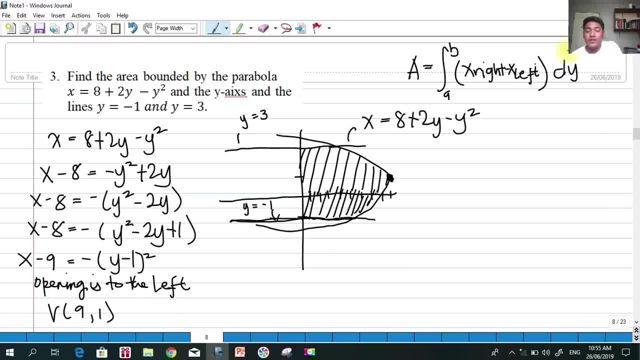 In this case, we will be needing a limits, that is, in terms of y, that's given from negative one to three. Okay, Now we're going to use the horizontal strip, So this will be our horizontal strip. okay, horizontal strip. 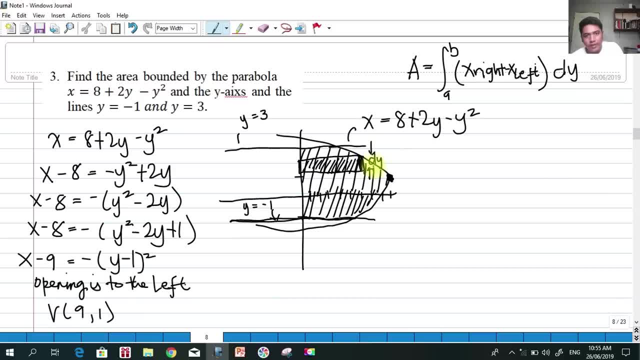 So this has a width of dy. Okay, And again the horizontal strip touches the other side. okay, on the other side, the parabola, And on the left side it touches the y-axis. So what will happen? Our x right would be actually what? 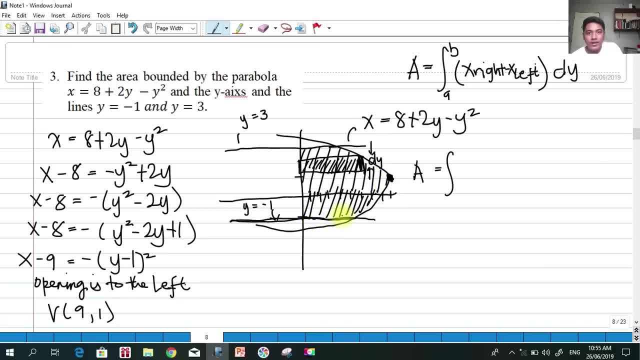 Our x right would be automatically the parabola. this parabola because it touches the parabola at the right side of the strip. So we have eight plus two y minus y squared minus x left. What would be our x left? 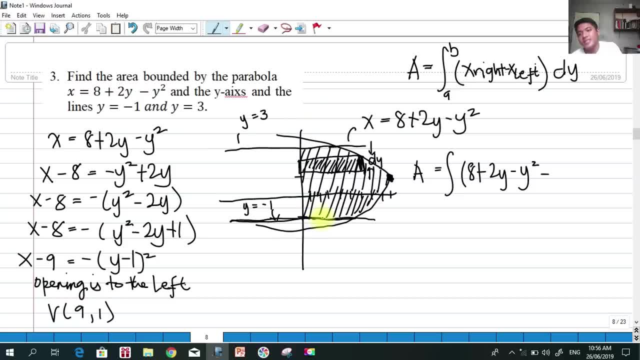 So the left side of the strip touches the y-axis, So that should be. that is not a curve, that is an axis, So that should be the y-axis. Okay, That should be zero. The y limits from negative one to three. 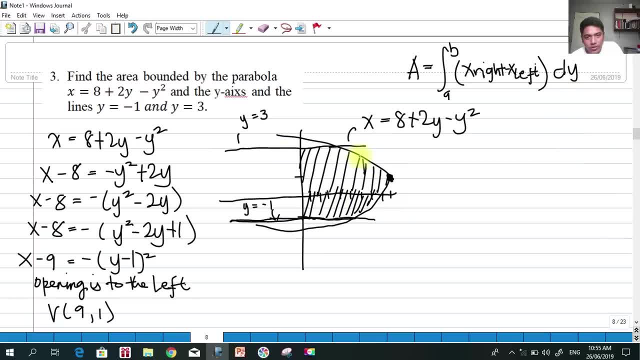 So we're going to use the horizontal strip, So this will be our horizontal strip, Okay, Horizontal strip. So this has a width of dy. Okay, And again, the horizontal strip touches the other side. okay, on the other side, the parabola. 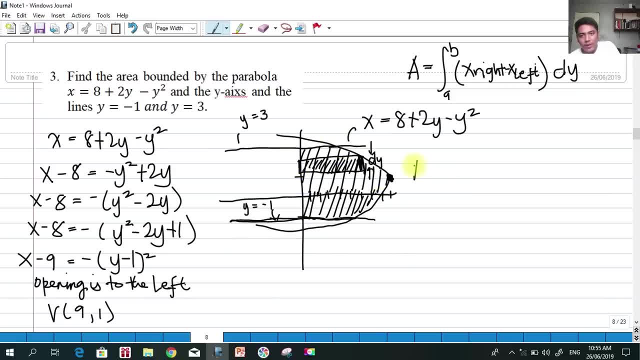 And on the left side it touches the y-axis. So what will happen? Our x right would be actually what Our x right would be automatically the parabola. this parabola because it touches the parabola at the right side of the strip. 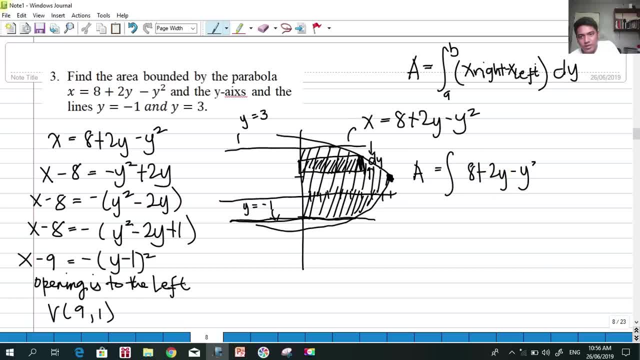 So we have 8 plus 2y, minus y squared minus x left. What would be our x left? So the left side of the strip touches the y-axis, So that should be. that is not a curve, that is an axis, so that should be 0.. 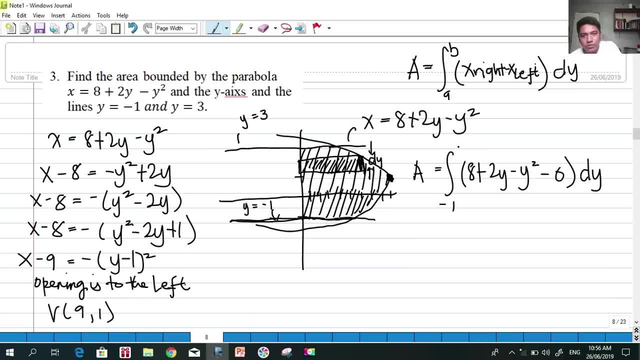 The y limits from negative 1 to 3.. It's given by the lines right. So if we integrate this, we'll be having what with respect to y? So we have 8y plus y squared, if I'm not mistaken. 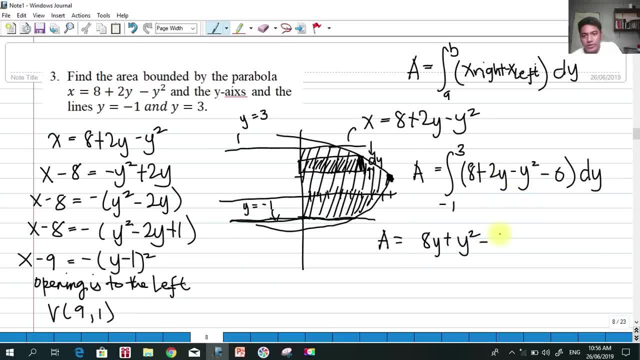 So 8y plus y squared, So 2y squared over 2, the 2s will cancel minus 1. third y cubed: okay. So evaluated from limits negative 1 to 3, okay, If we evaluate that we should be okay, as I have shown you a while ago. 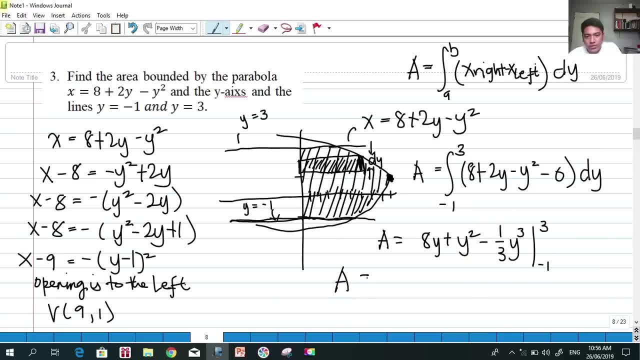 we will evaluate this definite integral, So our answer should be 92 over 3 squared Units. okay, So that should be our answer. Now the important thing here is you know how to graph the curve, the given curve. 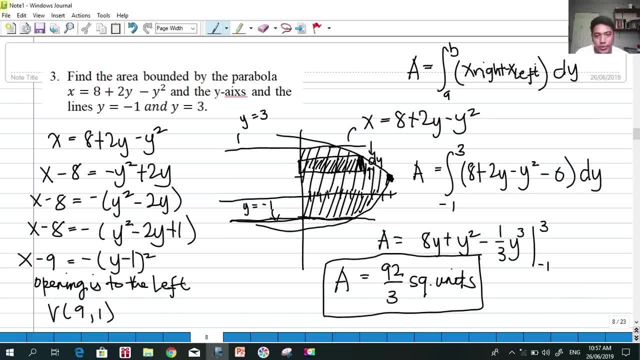 Then we're going to identify what strip are we going to use And of course, we have to identify the limits. And after identifying the limits, you have to perform now the integration. okay, So that is equivalent to 92 over 3 squared units. 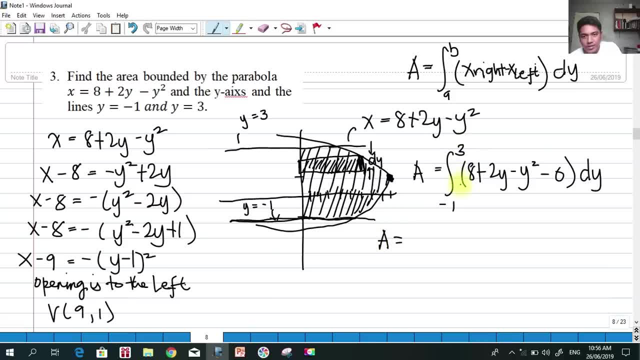 It's given by the lines right. So if we integrate this, we'll be having what with respect to y? So we have eight y plus y squared, if I'm not mistaken. So two y squared over two, the twos will cancel minus one-third y cubed. 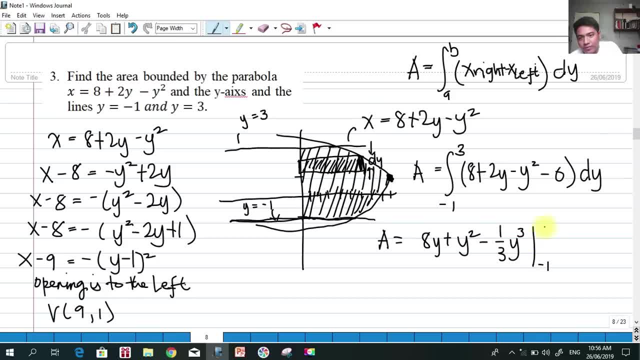 Okay. So, evaluated from limits, Negative: one, two, three. Okay, If we evaluate that we should be, as I have shown you a while ago, we will evaluate this definite integral. So our answer should be ninety-two over three square units. 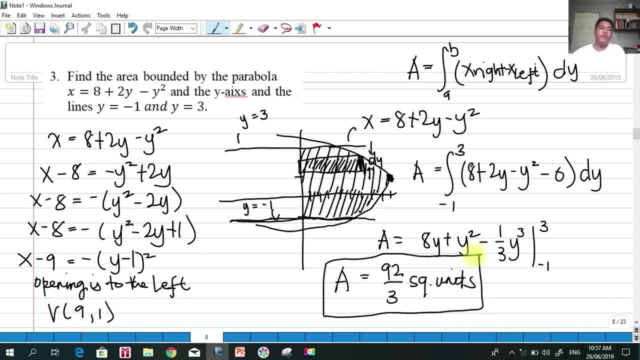 So that should be our answer. Now, the important thing here is: you know how to graph the curve, Okay, Okay, The given curve, The given curve. Then we're going to identify what strip are we going to use And, of course, we have to identify the limits. 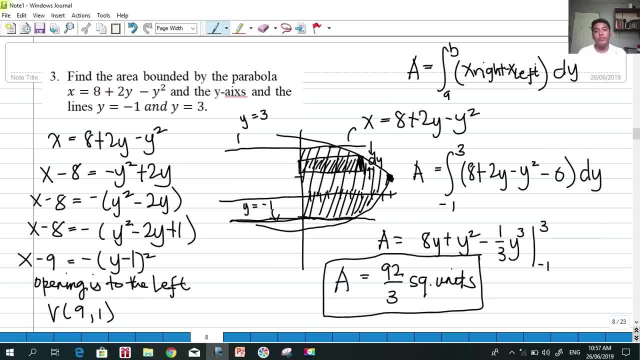 And after identifying the limits, you have to perform now the integration. Okay, So that is equivalent to ninety-two over three square units, And actually we have done an example wherein we have only one curve. Okay, So lines, A parabola and line. 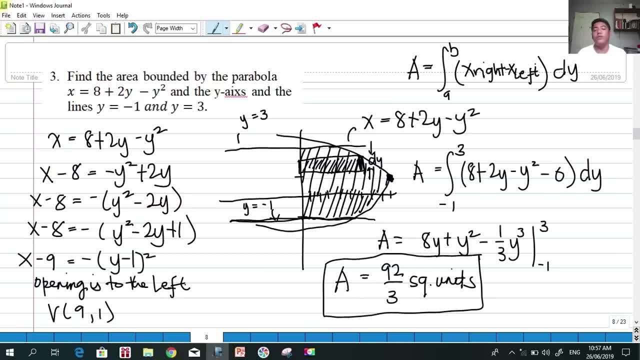 So what if we have a parabola and a line? Also, we're going to find the area of these two. And what if we have two parabolas? So it's also possible. Okay, For the next example, we'll have to try that. 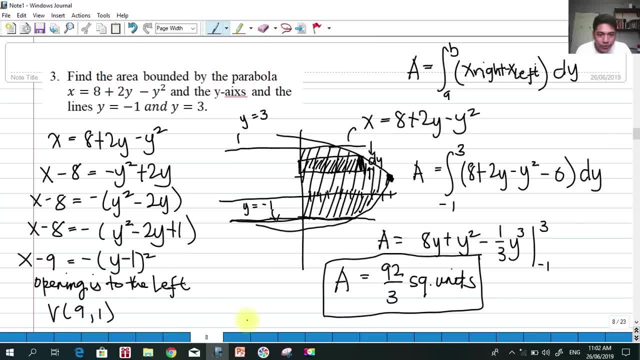 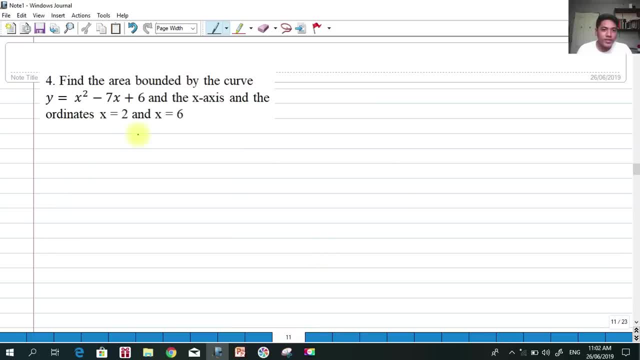 Okay, All right, So let's continue. For number four, we have find the area bounded by the curve. Okay, Y is equal to x squared minus seven, x plus six And the x axis and the x axis and the ordinance, x is equal to two and x is equal to six. 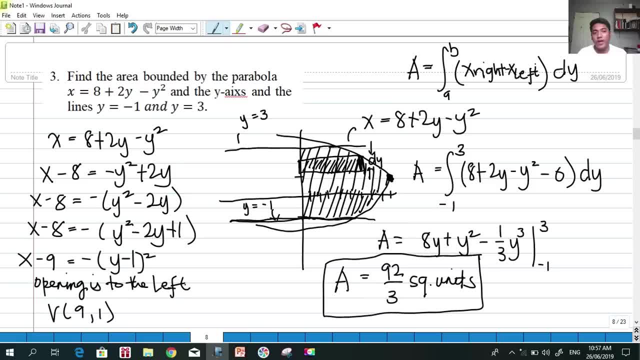 And actually we have done an example wherein we have only one curve. okay, So lines, a parabola and lines. So what if we have a parabola and a line? Also, we're going to find the area of these two. 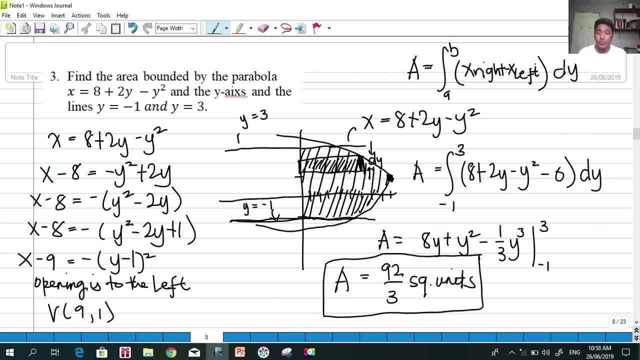 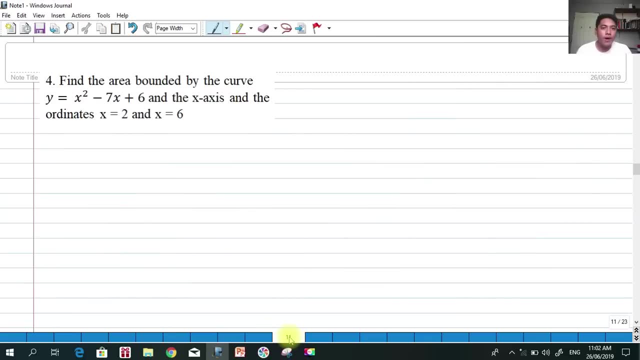 And what if we have two parabolas? So it's also possible. okay, For the next example, we'll have to try that. Okay, All right, So let's continue For number four. we have find the area bounded by the curve. 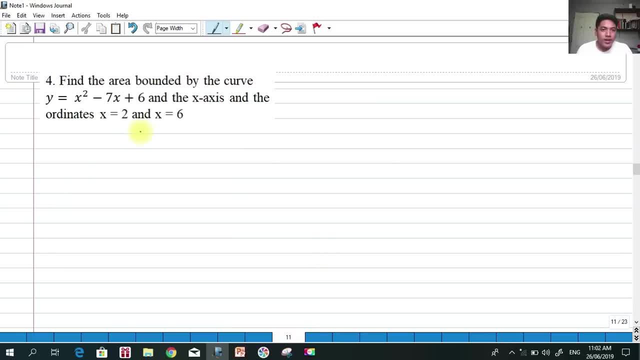 Y is equal to x squared minus 7x plus 6.. And the x-axis and the x-axis and the ordinance x is equal to 2 and x is equal to 6.. So again, they're the same problem, Okay. 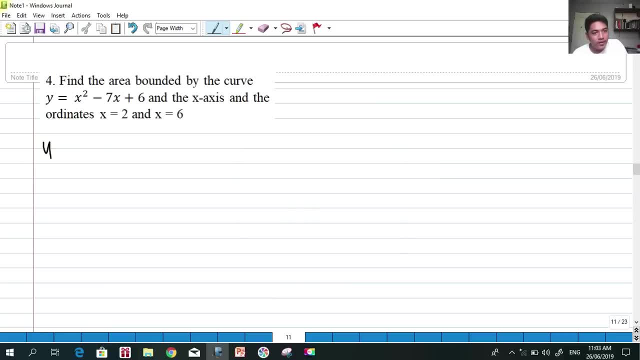 So we have to identify the vertices of this parabola So we can transpose 6 on the other side. So we have x squared minus 7x. Okay, So again we have to complete this square. x squared minus 7x, divided by 2, is 7 over 2.. 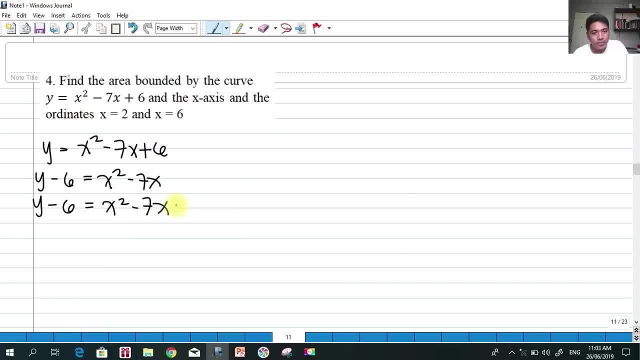 Okay, And we square that. So that must be last 49 over 4.. Okay, So if we add here, we have y minus 6 plus 49 over 4. Okay, And then we'll be having x minus 7.. 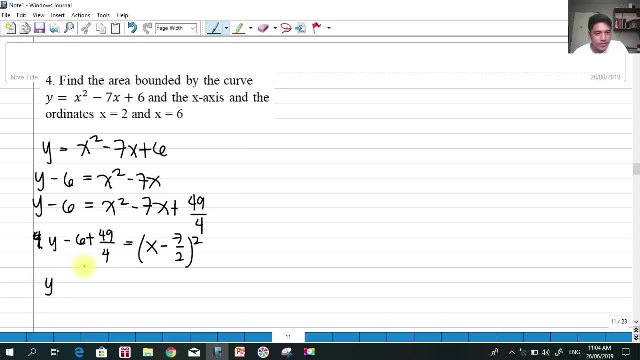 Okay, We can try to estimate the vertices of this. So minus 24.. Plus Plus 49 over 4. Okay, And we have x minus 7 halves squared, So we have 49 minus 23.. If I'm not mistaken, that is 23.. 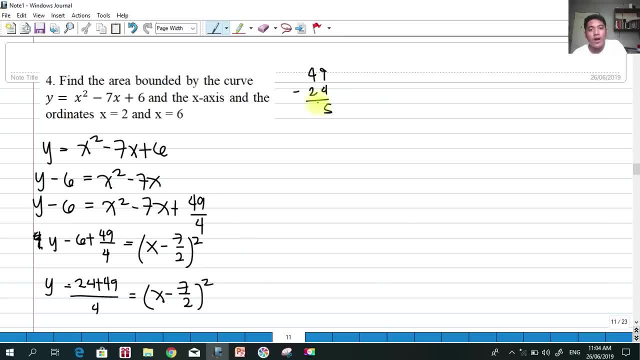 49 minus 24.. So we have 25.. Okay, So we have 25.. So that should be y minus or plus, Okay. 25 over 4 is equals to x minus 7, halves squared Okay. 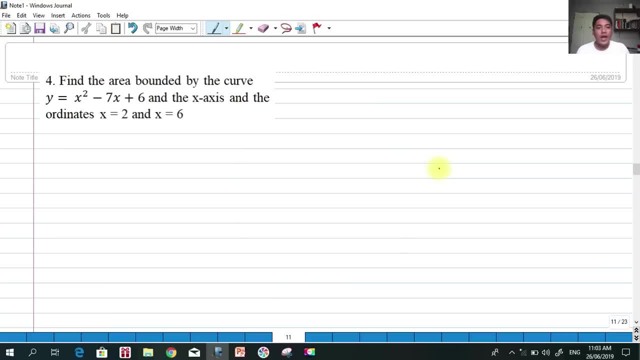 So again they're the same problem. Okay, So we have to identify the vertices of this parabola, So we get. Then transpose six on the other side, So we have x squared minus seven x. Okay, So again we have to complete this square. 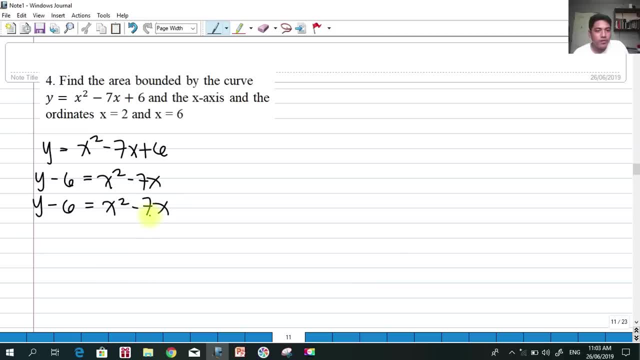 X squared minus seven, x divided by two is seven over two. Okay, And we square that, So that must be plus forty-nine over four, Okay. So if we add here, we have y minus six Plus forty-nine over four, Okay. 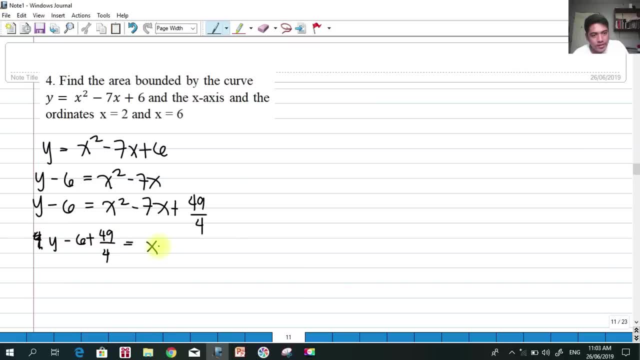 And then we'll be having x minus seven. We can try to estimate the vertices of this. So minus twenty-four plus forty-nine over four, Okay, And we have x minus seven halves squared, So we have forty-nine minus twenty-three, if I'm not mistaken. 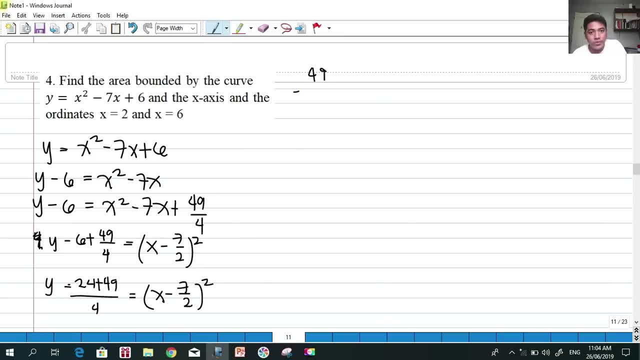 That is twenty-three, Forty-nine minus twenty-four, Twenty-five, Okay, So we have twenty-five. So that should be y minus or plus. twenty-five over four is equals to x minus seven, halves squared, Okay. So this is a parabola opening, but of course upward, with a vertex at the. let's say we: 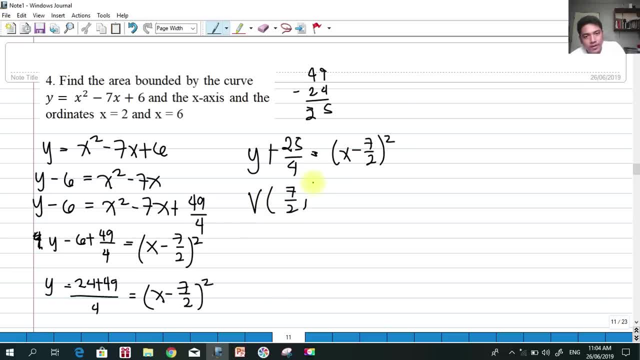 have a vertex at seven halves and negative twenty-five over four. So we can estimate that the parabola we are trying to solve is actually opening. This is an opening again upward. Okay, So it has a vertex of seven halves. 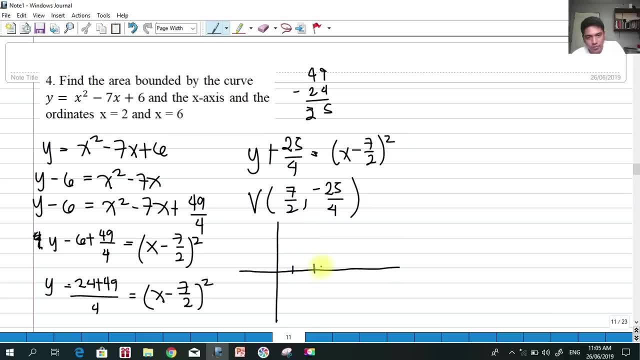 So seven halves is three point five. So we have one, two, three, Okay, And negative twenty-five over four. This should be approximately equal to four, eight, twelve, sixteen, twenty, thirty-four, Negative six point twenty-five, if I'm not mistaken. 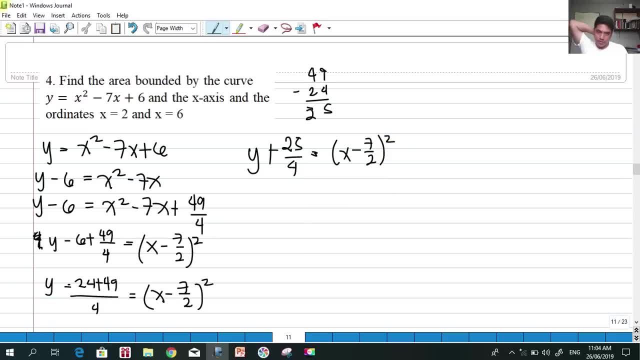 So this is a parabola opening, But of course upward, with a vertex at d. Let's say we have a vertex at 7 halves and negative 25 over 4. So we can estimate that the parabola 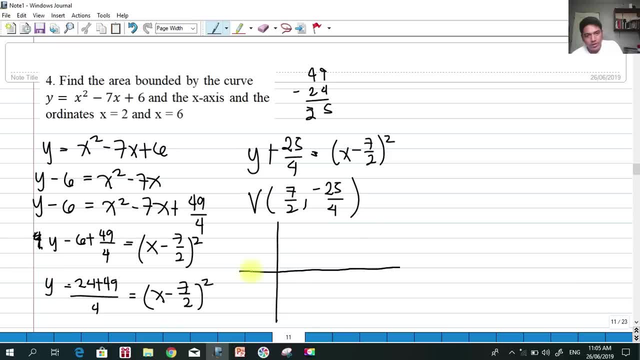 Okay. So what we are trying to solve is actually opening. this is an opening again upward, Okay. So it has a vertex of 7 halves. So 7 halves is 3.5.. So we have 1,, 2,, 3.. 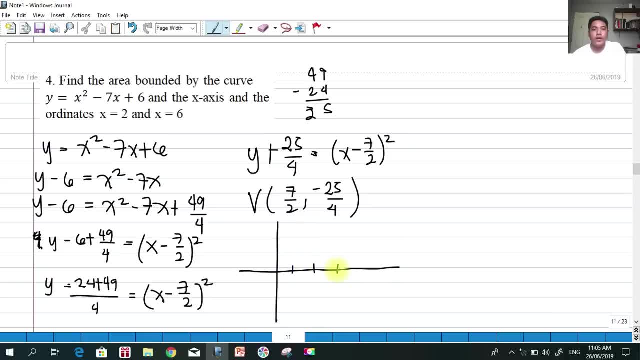 Okay, And negative: 25 over 4.. This should be approximately equal to 4, 8,, 12,, 16,, 20,, 34.. Negative: 6.25.. If I'm not mistaken, you know 2, 8,, 12,, 16,, 20,, 24.. 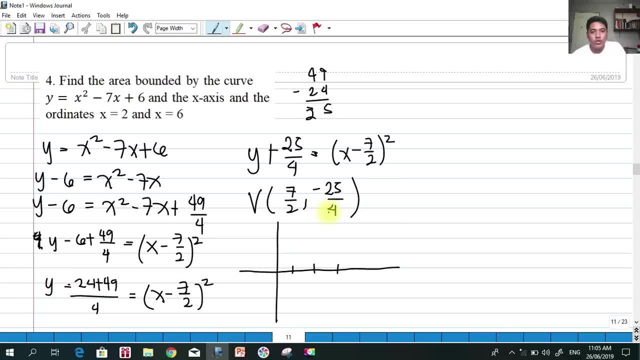 Negative 6.25.. If I'm not mistaken, you know 2,, 8,, 12,, 16,, 20,, 24.. Negative 6.25.. If I'm not mistaken, you know 2,, 8,, 12,, 16,, 20,, 24.. 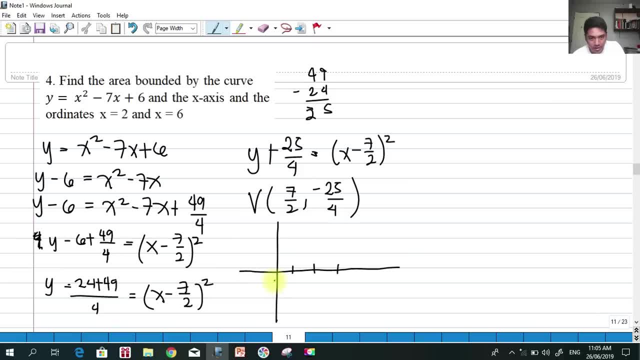 Negative: 6.25.. If I'm not mistaken, you know 2, 8,, 12,, 16,, 20, 24.. Negative: 2, 8,, 12,, 16,, 20,, 25.. 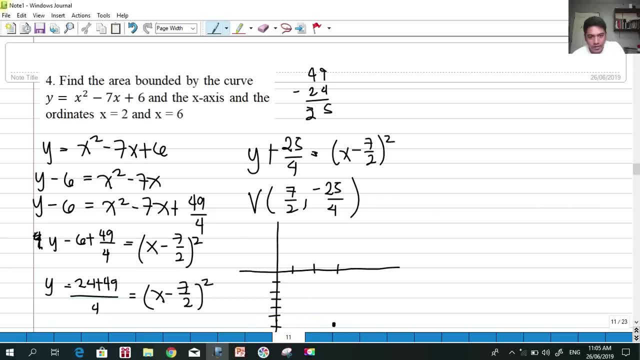 7,, 14,, 19,, 24.. Negative: 6.. Ok, let's say here: this is a rough graph of our parabola, So opening upwards. Well, as you can see, it passes this point, but we don't know exactly what that point. 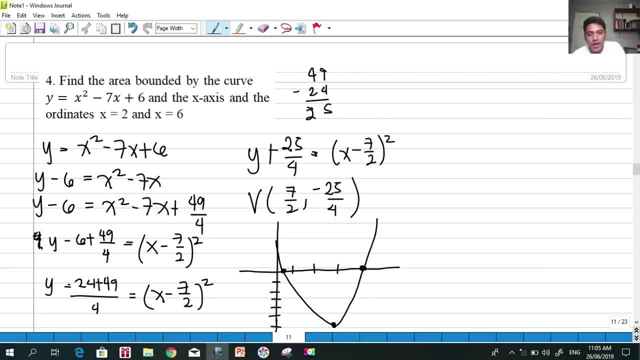 is, And carefully notice then that my drawing is not drawn to scale, Okay. So the point of interest is that the x-axis and the coordinates, okay, is equal to 2 and 6.. So if we're going to draw this, okay, so let's say this should be: our x is equal to 2, okay. 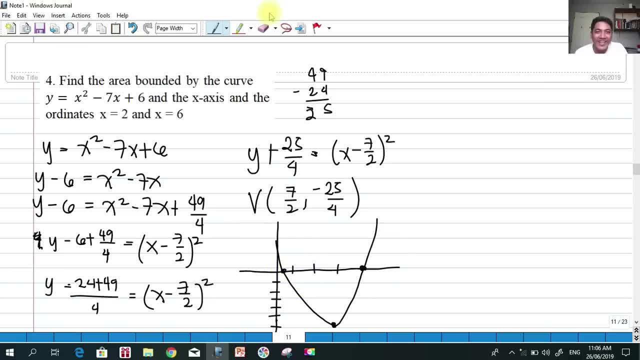 Let's say this is: let's draw again. okay, Let's draw again. Let's try to draw again. Okay, we have an ordinance equal to 2 and 6.. For example, if I'm going to draw this, okay. for example, here is our vertex of the parabola. 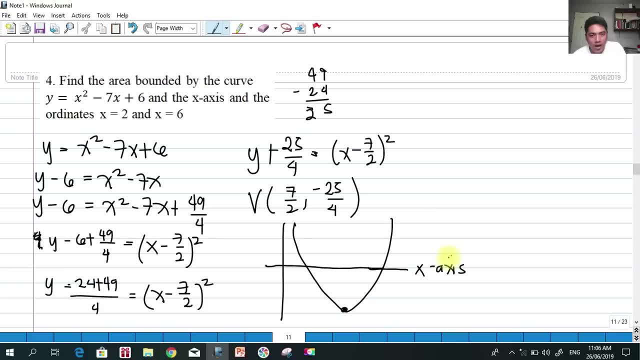 For example, let's say: this is x is equal to 2, okay, x is equal to 2.. And this is: x is equal to 6, okay, So the ordinance, x is equal to 2 and x is equal to 6.. 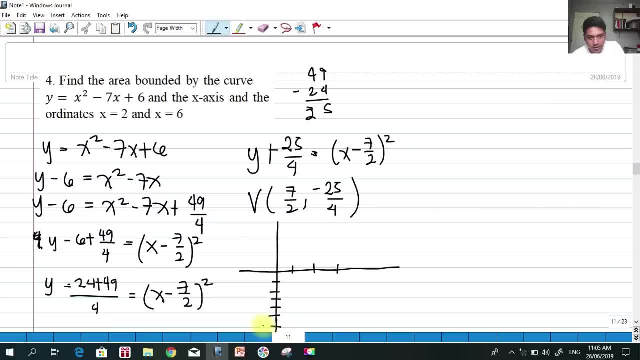 Two, thirty-three, four, five and negative six. Okay, Let's say here: This is a rough graph of our parabola, So, opening upwards, As you can see, it passes this point, but we don't know exactly what that point is. 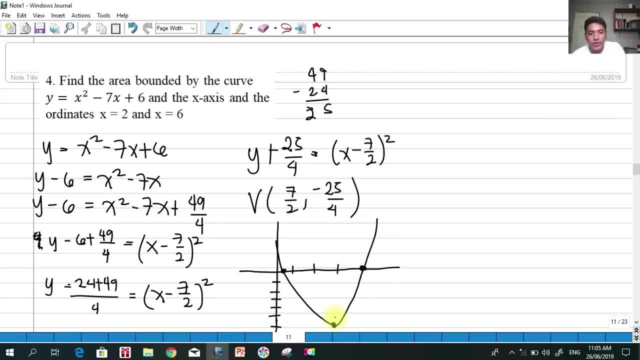 And carefully notice then that my drawing is not drawn to scale. So the point of interest is that the x-axis, and the ordinates, is equals to two and six. So If we're going to draw this, okay, so let's say this should be our: x is equals to two. 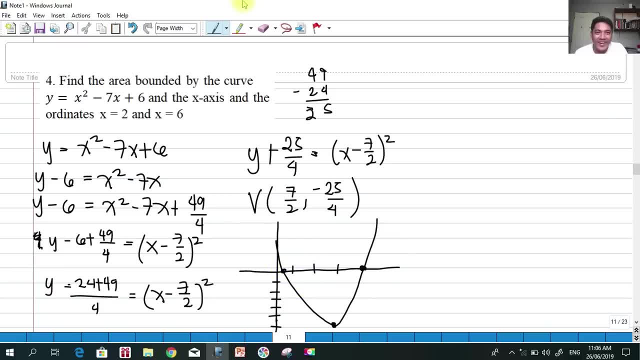 Okay, Let's say this is: Let's draw again. Okay, Let's draw again. Let's try to draw again. Okay, We have an ordinates equal to two and six. For example, if I'm going to draw this: 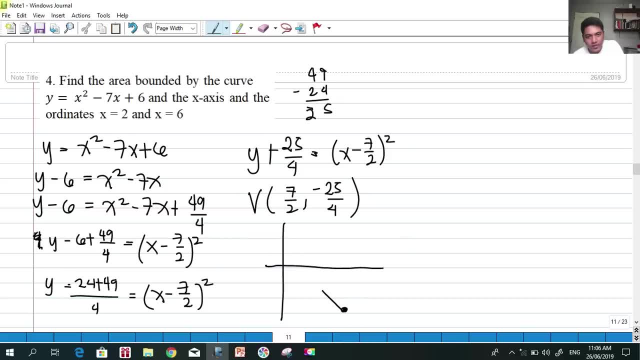 Okay, For example, here is our vertex of the parabola. For example, let's say: this is x is equals to two. Okay, x is equals to two. And this is x is equals to six. Okay, So the ordinates, x is equals to two and x is equals to six. 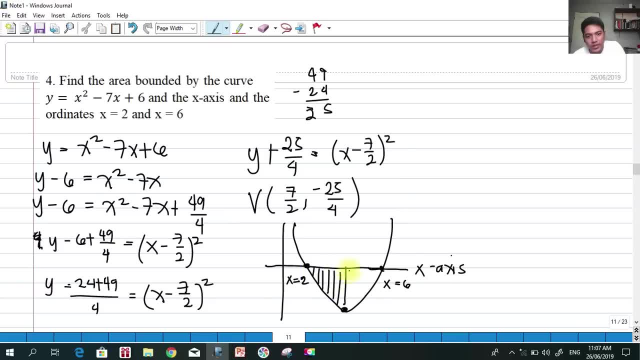 So the point of interest of our area should be this: Okay, And in this case, what are we going to use? So we are given a limit, So we are given a limit from x is equals to two and x to six. So from two to six. 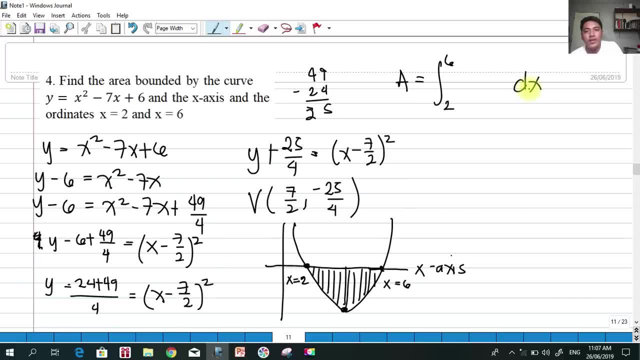 So we have to definitely use dx here. And what is that dx? If you use dx, we are going to use vertical strip. So y upper minus y lower. Okay, So here, if you use a vertical strip touching the upper part of the strip, so we have a. 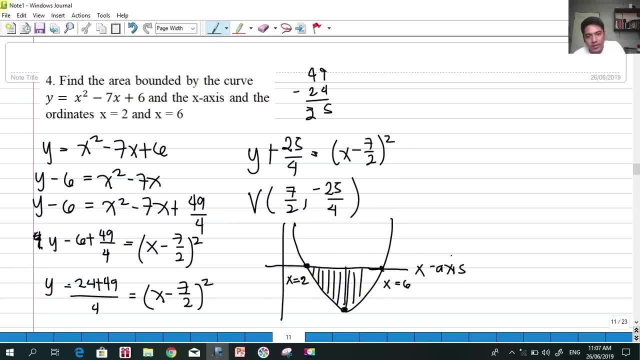 So the point of interest of our area should be this: okay, And in this case, what are we going to use? So we are given a limit: from x is equal to 2 and x to 6.. So, from 2 to 6.. 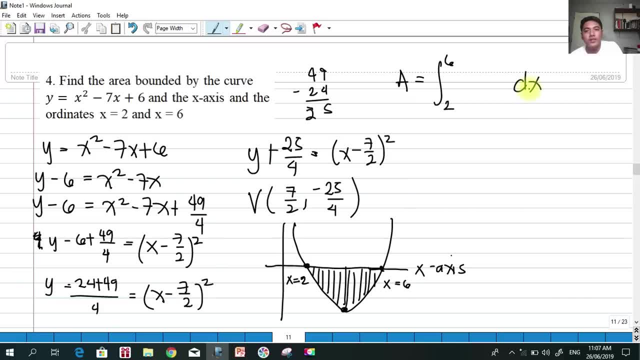 So we have to definitely use dx here. And what is that dx? If we use dx, we are going to use vertical slip, So y upper minus y lower. Okay, So here, if we use a vertical strip touching the upper part of the strip, 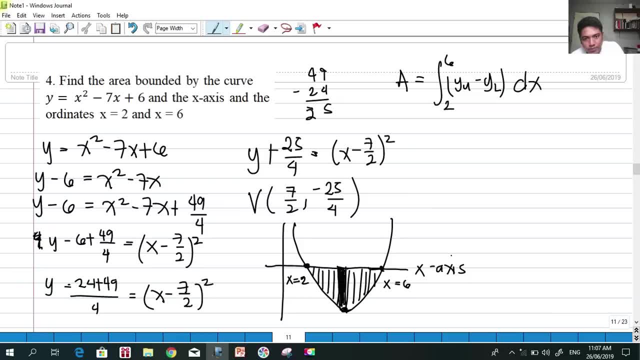 So we have a strip here, So our strip would be what does our strip touches? Okay, So we have a width of dx here, So upper, its upper, touches the x-axis. So our y upper should be what? 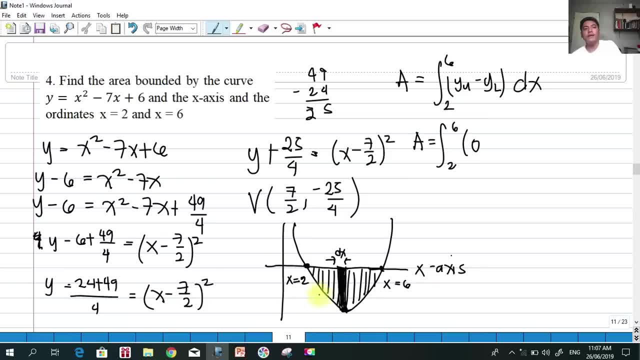 Should be 0. Our y lower touches, So our y lower touches, the parabola. So that should be negative of the x squared minus 7x plus 6 dx And of course, if we evaluate that So we have from 2 to 6.. 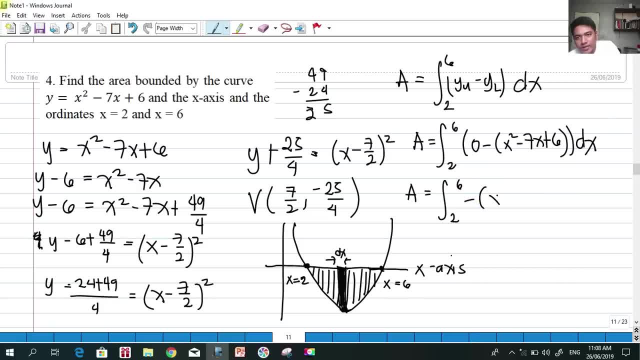 We have the integral of the negative of x squared minus 7x plus 6.. Okay, So dx. So simply, if we integrate this, we have the negative of the 1 third of the x cubed minus 7 halves of the x squared plus 6x evaluated from 2 to 6.. 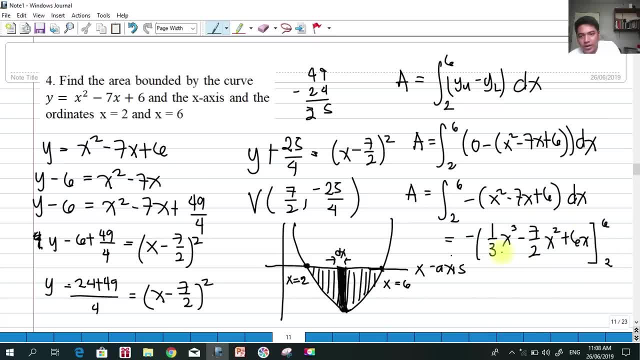 If you evaluate this, we're going to evaluate this. So your answer should be equal now to 56 over 3 squared. So if you evaluate this, you're going to get 56 over 3 squared units. Take note that it's okay to have a negative here, because actually that is the equation: y upper minus y lower. 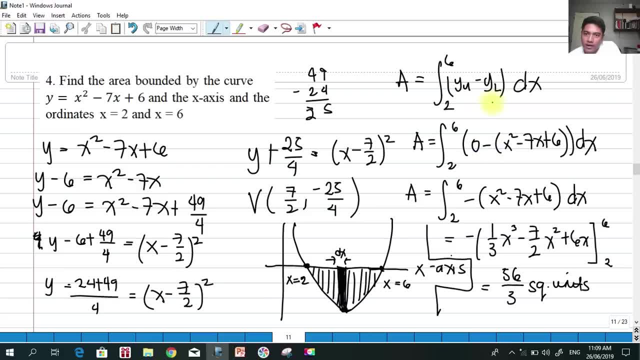 And we have a negative here, because the y lower is now the parabola. Okay, So if you evaluate this definite integral with the negative, it should give you 56 over 3 squared units. Okay. So let's try another example. 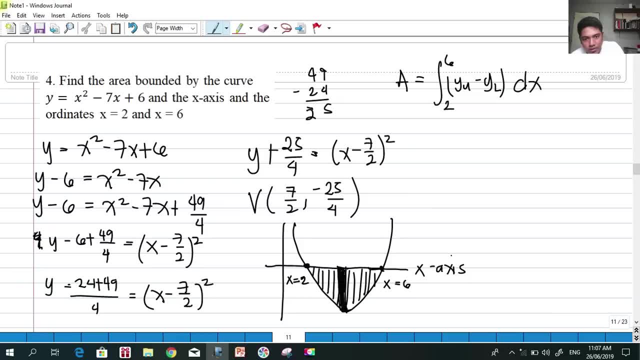 strip here. Okay, So our strip would be. what does our strip touches? Okay, So we have a weight of dx here. So upper, its upper touches the x axis. So our y upper should be what Should be zero, Our y lower touches the parabola. 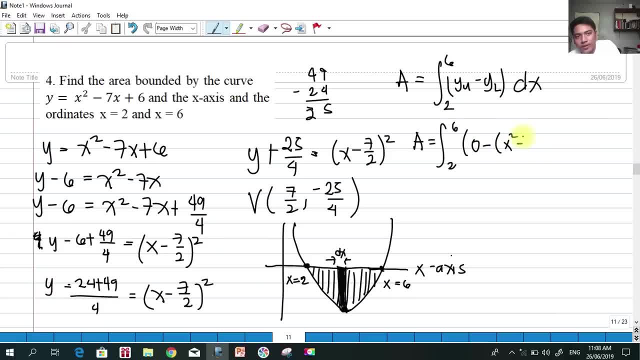 So that should be negative of the x squared minus seven, x plus zero. Okay, So we have a negative of the x squared minus seven, x plus six, dx, And of course, if you evaluate that, so we have from two to six, We have the integral of the negative of x squared minus seven, x plus six. 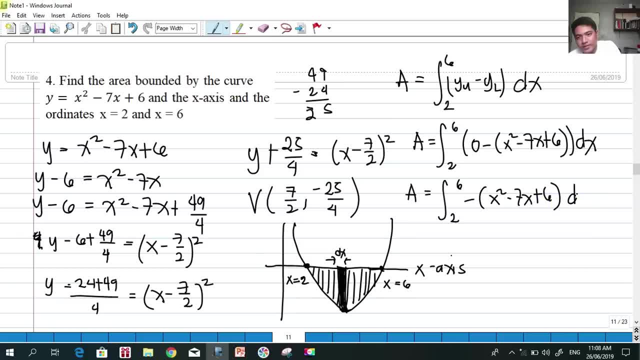 Okay, So dx. So simply, if we integrate this, we have the negative of the one-third of the x cubed minus seven hundred and fifty-eight. Okay, of the x squared plus 6x, evaluated from 2 to 6, if you evaluate this as you're. 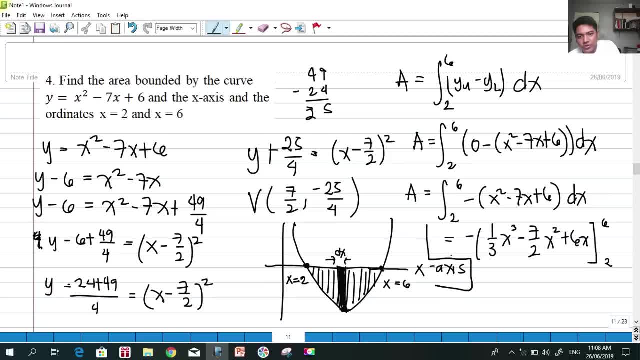 going to evaluate this. so your answer should be equal now to 56 over 3 square units. take note that it's okay to have a negative here, because actually that is the equation y upper minus y lower. and we have a negative here because the y lower is now the parabola okay. so if you evaluate this definite integral with the 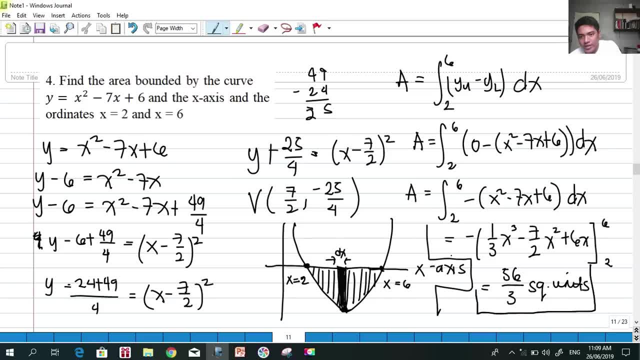 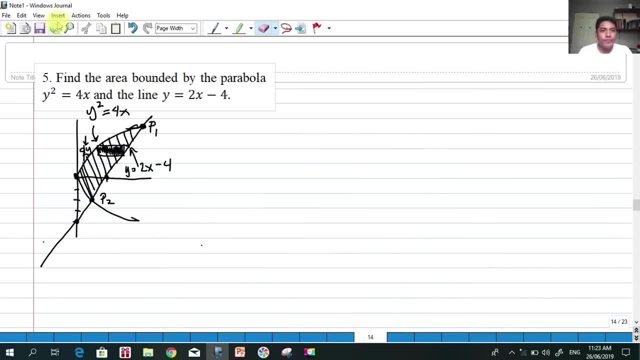 negative, it should give you 56 over 3 square units. okay, so let's try another example. so here we have already a drawing. a find: the area bounded by the parabola y squared is equal to 4x and the line y is equal to 2x minus 4. as you can see, here we have already graphed the 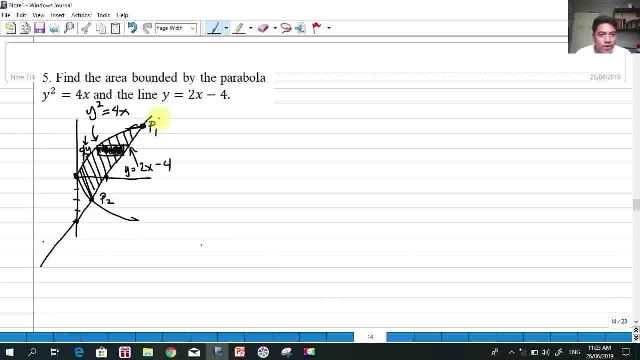 parabola and the line. this is the line 2x minus 4, and this is the parabola with a vertex of 0, 0 opening to the right. so, as you can see, we need to use the horizontal strip. you can either use vertical or horizontal here, but it's much easier to. 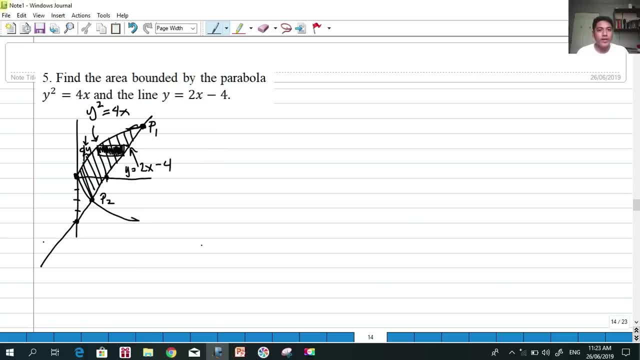 So here we have already a drawing. Find the area bounded by the parabola. y squared is equal to 4x And the line y is equal to 2x minus 4.. As you can see, here we have already graphed the parabola and the line. 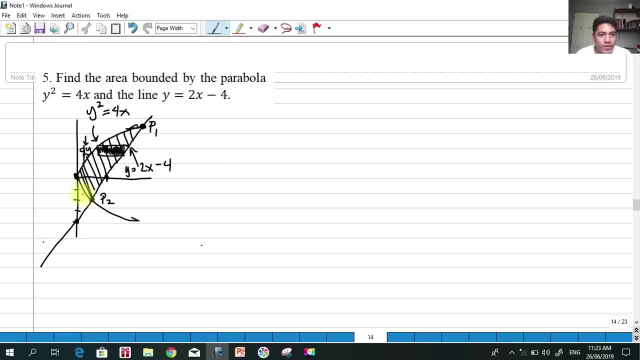 This is the line 2x minus 4.. And this is the parabola, with the vertex of 0, 0 opening to the right. So, as you can see, we need to use the horizontal strip. We can either use vertical or horizontal here. 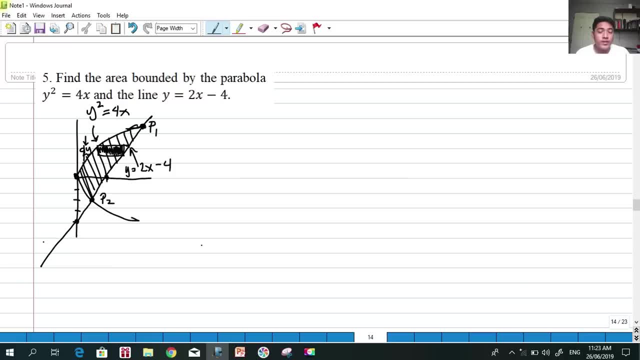 But it's much easier. It's much easier to use the horizontal strip here. Okay, So what are we going to do? First, we have already graphed the line and the parabola, So we used horizontal strip. So what are we going to do? here is what. 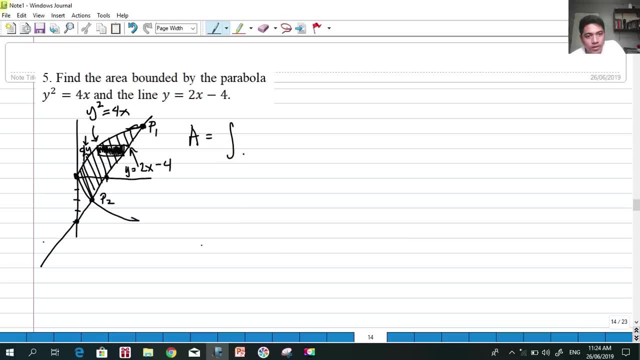 So we have: area is equal now to the integral from a to b. Since we used horizontal, that is x right minus x left. Okay, So we have to express this equation, these two equations: y squared is equal to 4x and y is equal to 2x minus 4, both in terms of x. 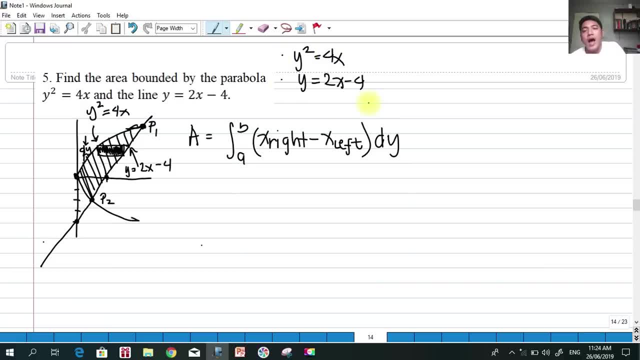 We're going to isolate x here for the first equation, and the second equation isolate x. So if we do that, so we have now: x is equal to 1, fourth y squared. And here we have: x is equal to y plus 4.. 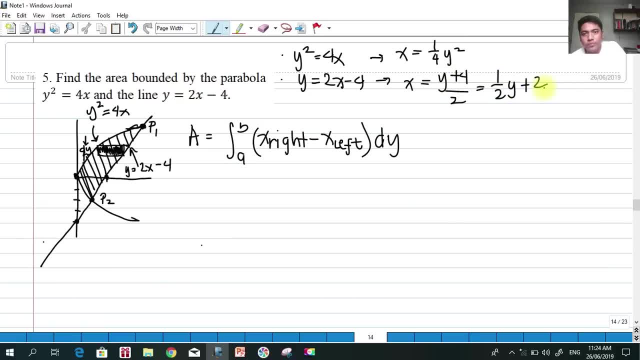 4 over 2, that should be 1 half y plus 2.. Okay, And we have now the formula. The problem is, we don't know the limits. So, as you can see here, the strip is drawn here. So we have what. 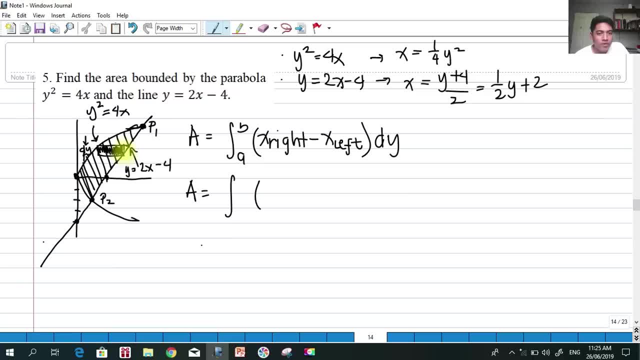 The x right, touching the rightmost of our strip, is the line. So that should be our x right's line. So it's our equation. This is our equation for the line. So we have 1 half y plus 2.. 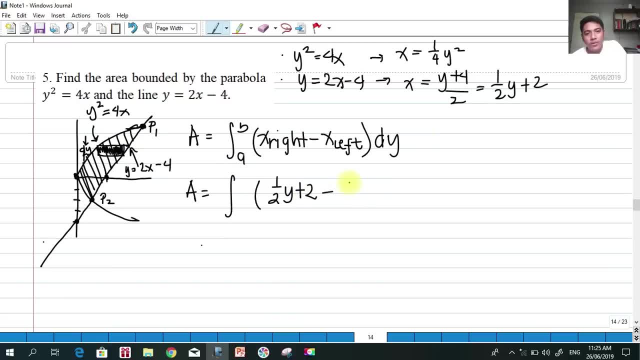 Minus, of course, the x left touches the parabola, which is 1 fourth y squared. okay, dy, And the problem is: what are the units? Okay, in order for us to get the units first, we have to what? 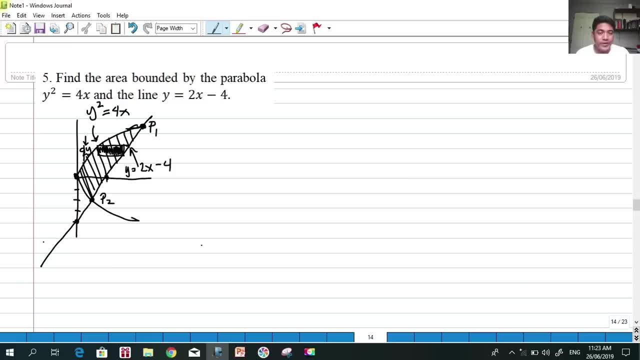 use the horizontal strip here, okay, so what are we going to do? first, we have the parabola, so we used horizontal strip. so what are we going to do here? is what? so we have, area is equals now to the integral from a to b. since we use 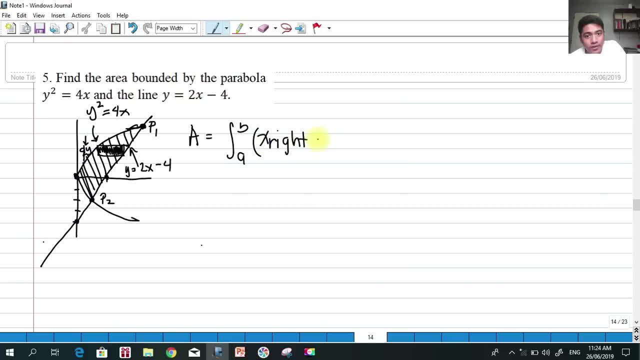 horizontal, that is x right minus x left. okay, dy, okay. so we have to express this equation, this two equation: y squared, this equals 4x and y squared is equal to 1 and dy will be equal to 0, because respect, the integral, is equal to 2x minus 4, both in terms of x. we're going to isolate x here for the first equation. 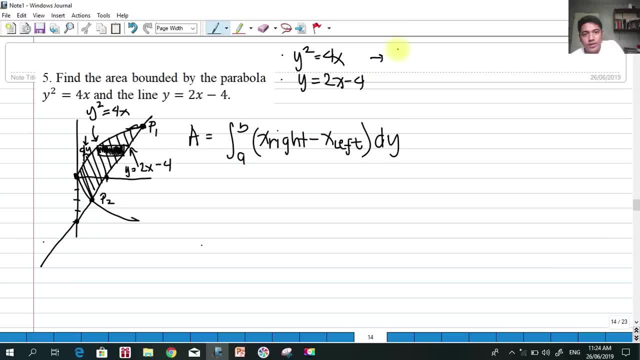 and the second equation isolate x. so if we do that, so we have now: x is equal to 1, 4 y squared. and here we have, x is equal to uh, y plus 4 over 2. that should be 1 half y plus 2, okay, and we have. 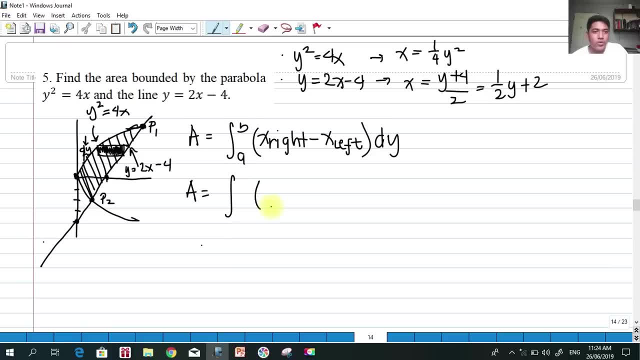 now the formula. the problem is we don't know the limits. so as you can see here the strip is drawn here. so we have what the x right touching the right most of our strip is the line. so that should be our x right line. so it's our equation. this is our equation for the line. so we have 1 half. 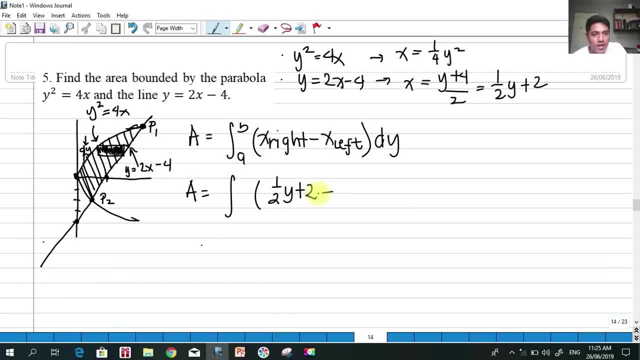 y plus 2 minus. of course, the x left touches the parabola, which is 1: 4 y squared. okay, dy, and the problem is: what are the units? okay, in order for us to get the units first, we have to what we have? to equate these two. okay, we have to equate these two, or we have, we can. 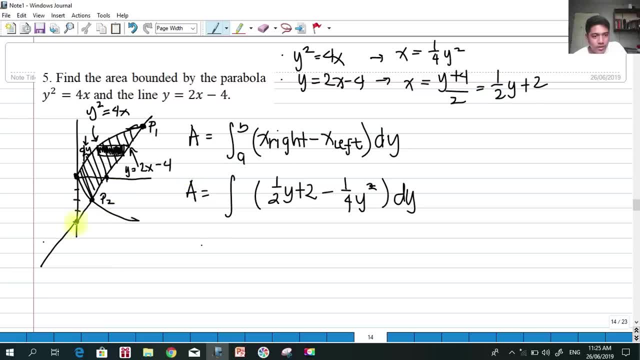 equate also these two. so, but we'll try to equate: y, squared is equal to 4x and y is equal to 2x minus 4. okay, equate that so by simply 2x minus 4 squared so equals to 4x. so if we're going to solve that, so we have 4x squared minus 16x plus 16 is equals. 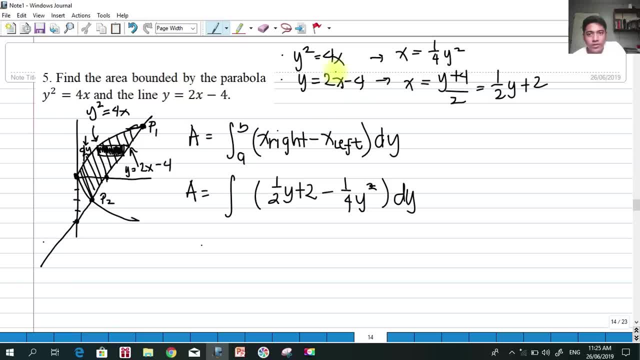 We have to equate these two. okay, We have to equate these two, or we can equate also these two. So, but we're trying to equate. y, squared is equal to 4x and y is equal to 2x. 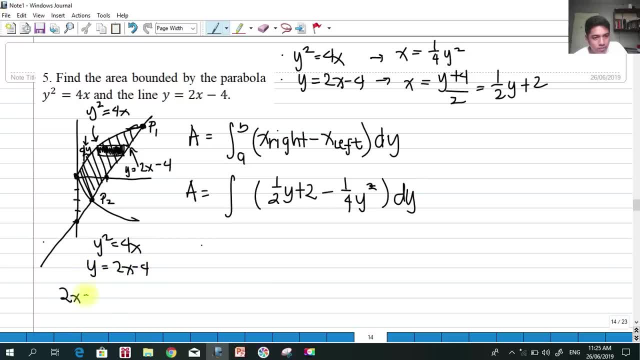 Minus 4.. Okay, let's equate that So by simply 2x minus 4 squared So equals to 4x. So if we're going to solve that, So we have 4x squared minus 16x plus 16 is equal to 4x. 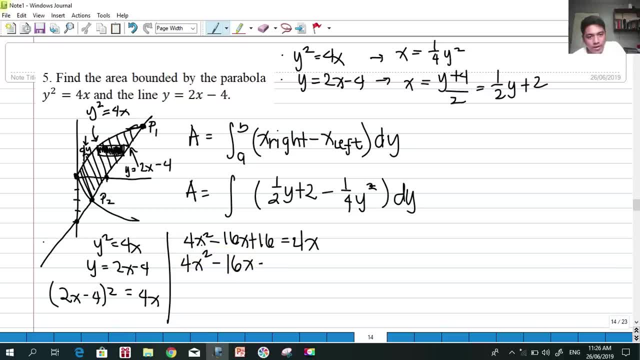 Transposing 4x. on the other side, we have minus 4x. here plus 16 is equal to 0. So we have 4x squared minus 20x. Plus 16 is equal to 0. And we can divide this whole equation by 1 over 4.. 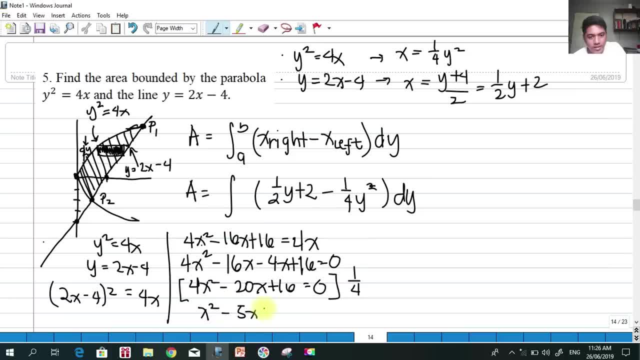 So that we have x squared minus 5x plus 4 is equal to 0.. So we can factor out this: So we have x minus 1 and x minus 4 is equal to 0. So in other words, the x intersection is: x is equal to 1 and x is equal to 4.. 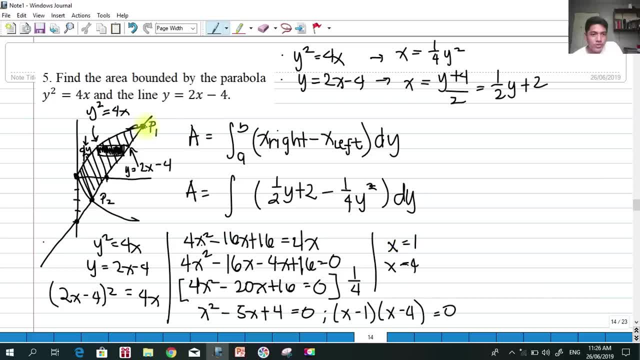 So these are not the The points of intersection in the x coordinate of this one. So this would be 4.. Okay, That is for sure. The coordinate x coordinate of that is 4.. And the coordinate of this second point of intersection is: 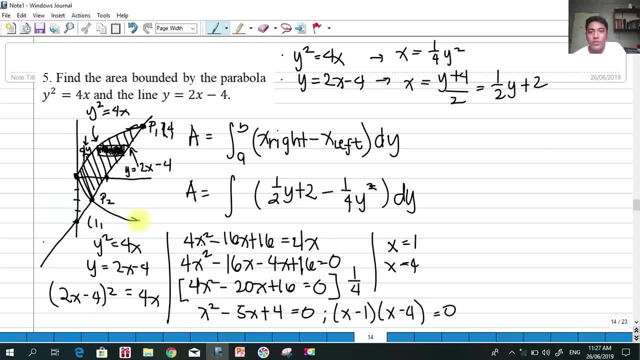 Well, actually it's 1. We don't know the y, So we are concerned to get the y, because our limits here from a to b should be in terms of y. And what are we going to do? How are we going to do that? 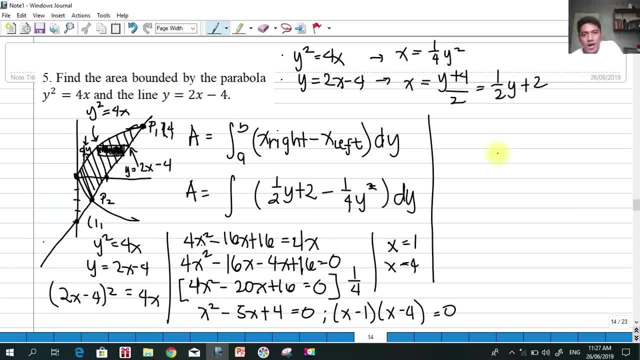 So simply choose one of Regulation. Let's say I choose. y is equal to 2x minus 4. And we're going to insert the roots that we get. So first is 1. 2 times 1 minus 4.. 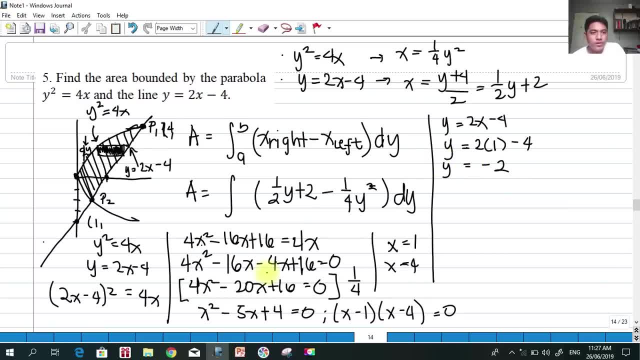 So 2 minus 4 is negative 2.. So there is a point of intersection, that it is negative 2.. And it is evident that this is 1 and negative 2.. So my drawing is not drawn to scale. 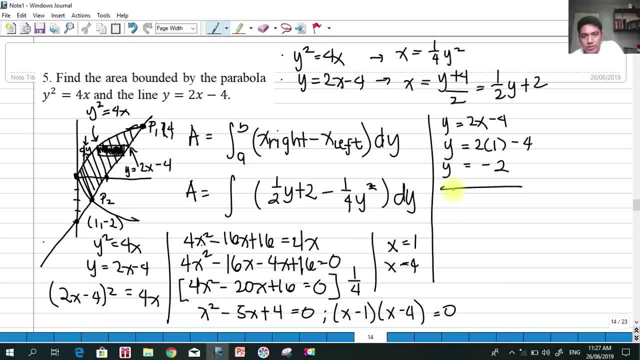 Okay, So, and of course, if we're going to Insert, y is equal to, let's say, 4. 4 times 2 here, 4 times 2, because 2x minus 4 minus 4.. You have 8 minus 4.. 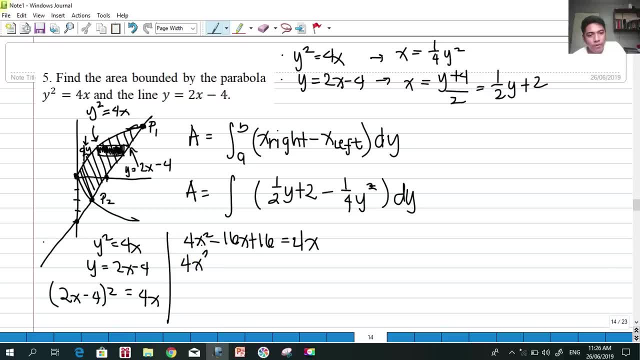 to 4x. transposing 4x on the other side, we have minus 4x. here. plus 16 is equals to 0, so we have 4x squared minus 20x. plus 16 is equals to 0 and we can divide this whole equation by 1. 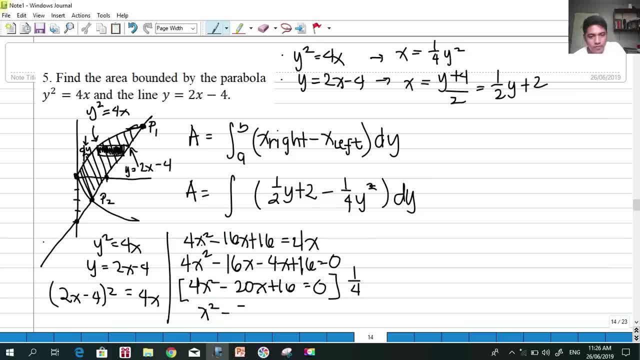 so we're going to get 4x squared minus 15x plus 16 is equals to 4, so that we have x squared minus 5x plus 4 is equals to 0. so we can factor out this so we have x minus 1 and x minus 4 is equals to 0. so in other 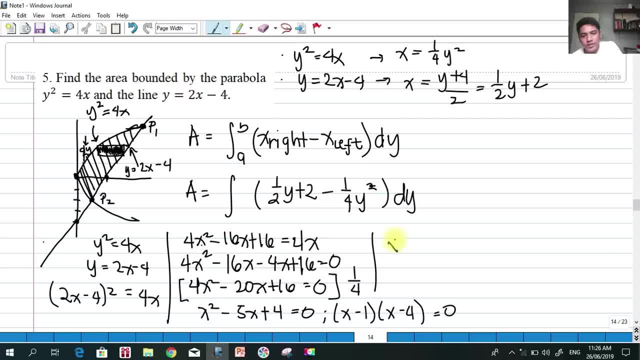 words, the x intersection is: x is equals to 1 and x is equals to 4. so these are not the. these are the points of intersection in the x coordinate of this one. so this would be 4 and this would be 4. Okay, That is for sure. The coordinate x, coordinate of that, is 4.. And the coordinate of this second: 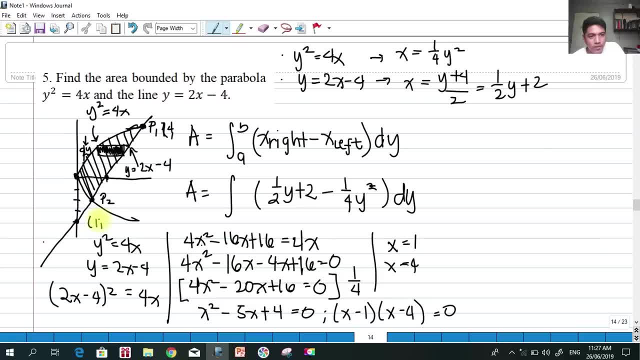 point of intersection is: well, actually is 1. We don't know the y, So we are concerned to get the y, because our limits here, from a to b, should be in terms of y. And what are we going to do? How? 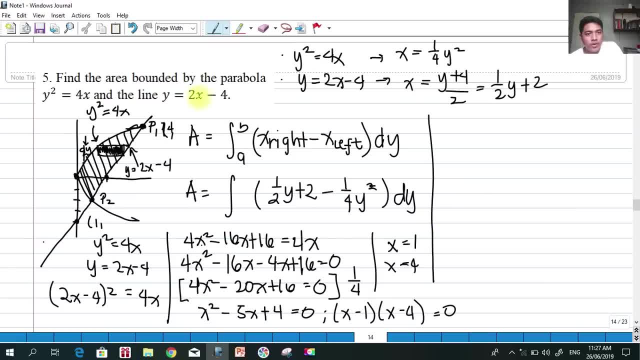 are we going to do that? So simply choose one of the equation. Let's say I choose y is equals to 2x minus 4.. And we're going to insert the roots that we get. So first is 1, 2 times 1 minus 4.. 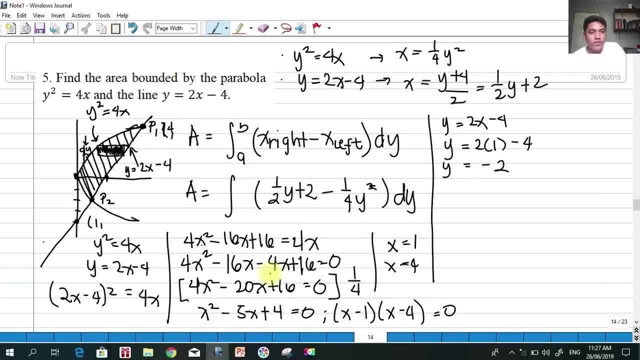 So 2 minus 4 is negative 2.. So there is a point of intersection that it is negative 2 and it is evident that this is 1 and negative 2.. My drawing is not drawn to scale And, of course, if we're 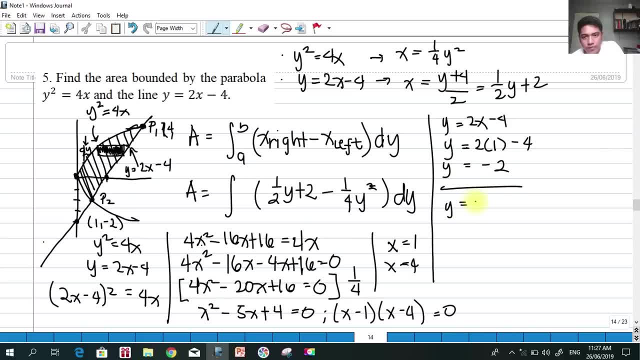 going to insert y is equals to, let's say, 4. 4 times 2 here. 4 times 2 because 2x minus 4 minus 4. You have 8 minus 4.. That should be equal to. 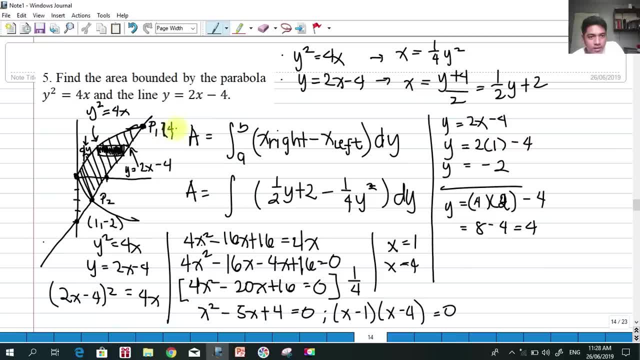 4.. So I can say that this is also 4.. So our concern now is the y coordinate of the point of intersection. So we have from negative 2 to 4. So from negative 2 to 4. So that will be our limit.